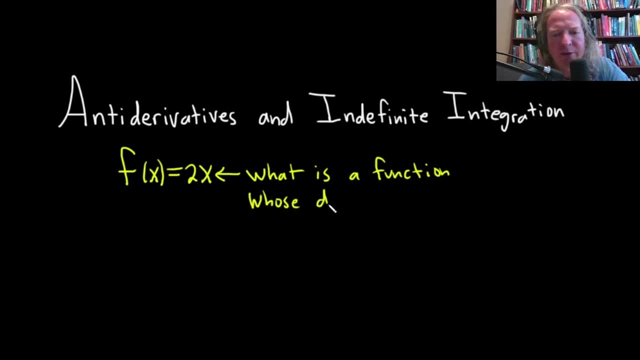 whose derivative is 2x. Whose derivative is 2x? And it's a pretty easy question. If you already know calculus, you might say: x squared right, x squared is an example of a function whose derivative is 2x, because you can bring the two down and you can subtract one from the exponent. 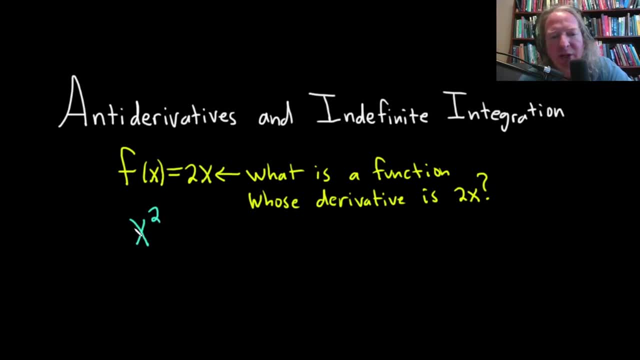 and basically just applying the power rule and you'll get 2x. I'm going to give this a name, I'm going to give it a name, and I'm going to give it a name, and I'm going to give it a name. 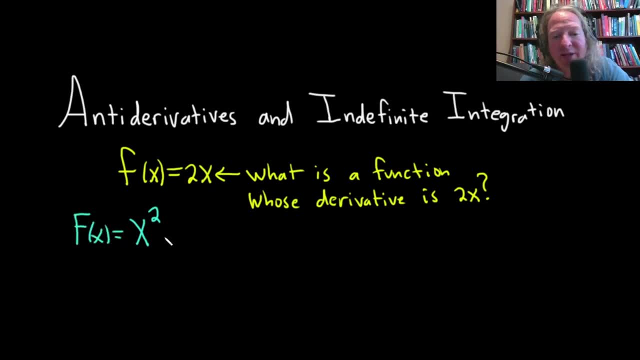 I'm going to give it a name, and I'm going to give it a name, and I'm going to give it a name, and I'm going to call it big f of x. And this is an example of what's called an antiderivative. 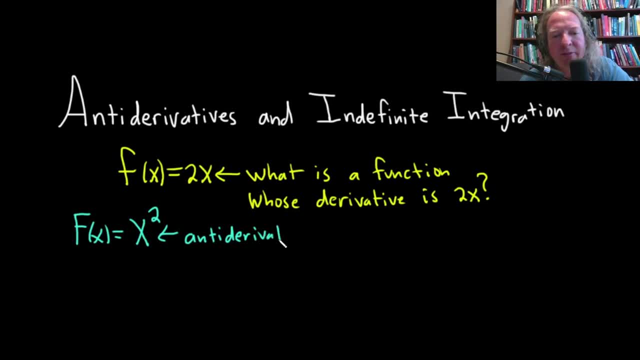 So this is an antiderivative. So we would say that x squared is an antiderivative for 2x, because the derivative of x squared is equal to 2x. So the thing is, there's other possible answers. For example, let's say I say big f of x is equal to x squared plus 1.. 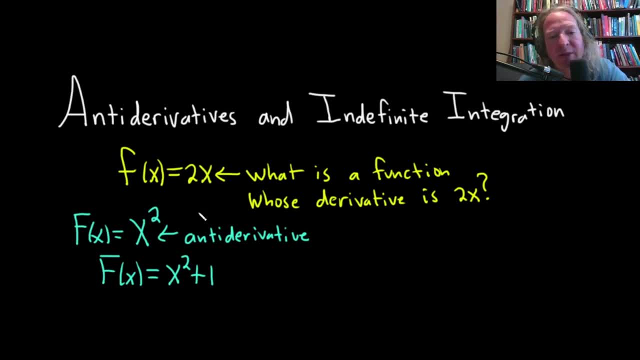 Well, if you take the derivative here, you're going to get the same thing. You're going to get 2x. The derivative of x squared is 2x and the derivative of 1 is 0. So you're going to get. 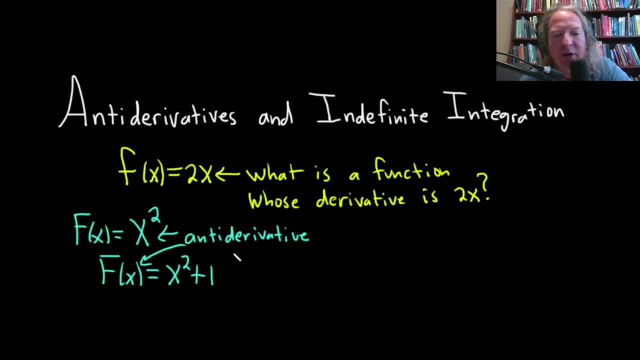 the same answer, But this is also an antiderivative for 2x. In fact, we can look at big f of x and call it x squared plus any number. I'll use a capital C, And this is also an antiderivative. 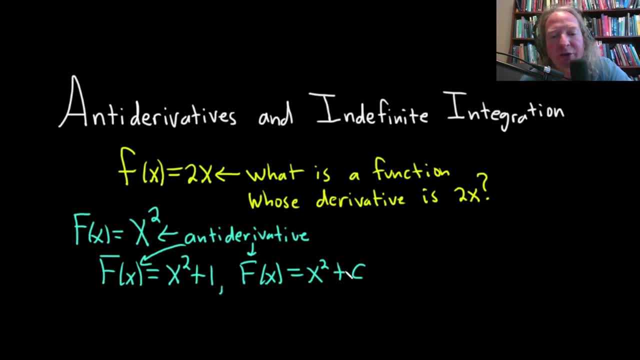 for 2x. This one has a name, This one's called the general antiderivative And this C. here it's an arbitrary constant. That's the word we often use, Arbitrary constant. So it could be any number, We don't know. That's an R there, Arbitrary. This is hard to read. 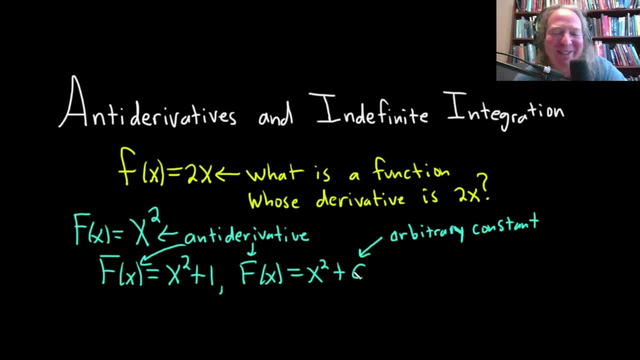 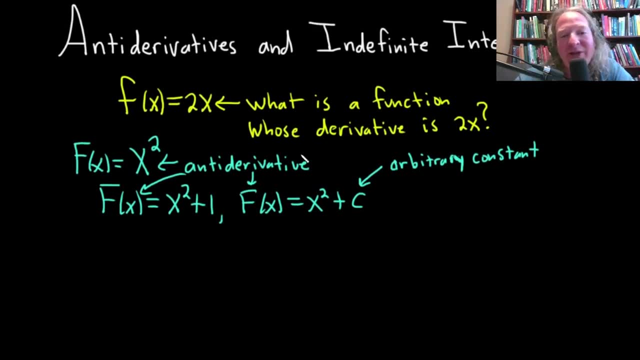 So A-R-B-I-T-R-A-R-Y Arbitrary constant. So there's infinitely many antiderivatives for 2x. Let me just go ahead and give you the definition. so you have it in place. So we say a function. 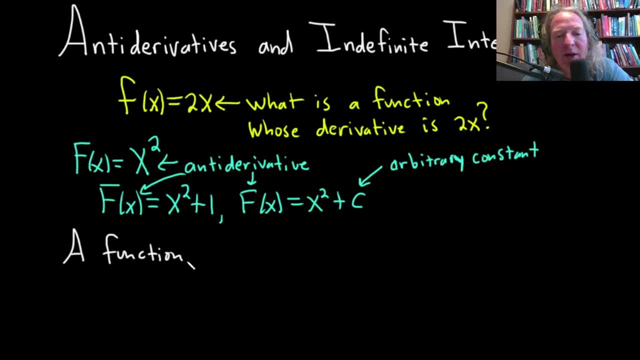 big F is an antiderivative, So antiderivative of little f, on some interval i. So I'll say on an interval i. So that's, when you take the derivative of big F It's equal to little f. And this is true for all x in your intervals, So for all x in i's. 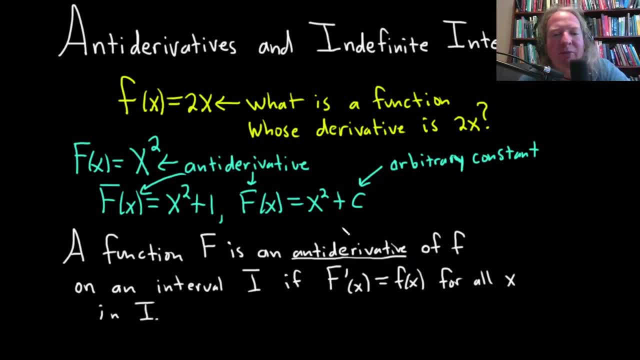 That's the definition of an antiderivative and typically in a calculus class you do use this, but in the actual problems that you do in calculus you don't use it too much. This would come up a little bit more in, maybe, a proof based class or something like that. 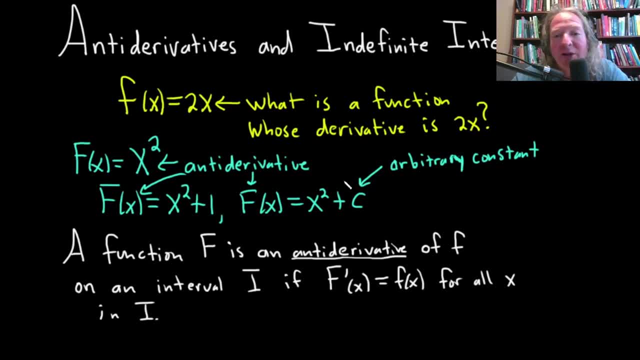 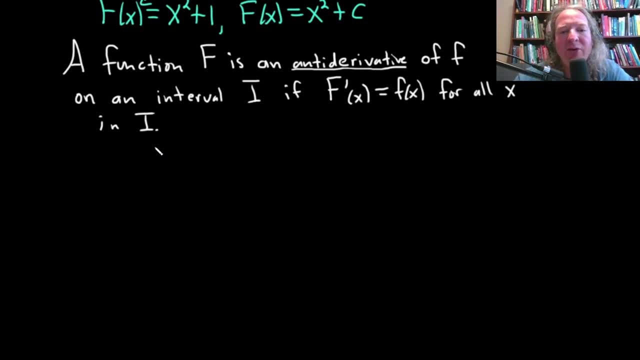 infinitely many. right, there's infinitely many. and now let's talk about what integration is, and I'm going to give you the notation. I'm going to switch colors here. oh, before I do, though, let's actually do it with respect to this example, so that way it doesn't look so abstract. so here's the notation that. 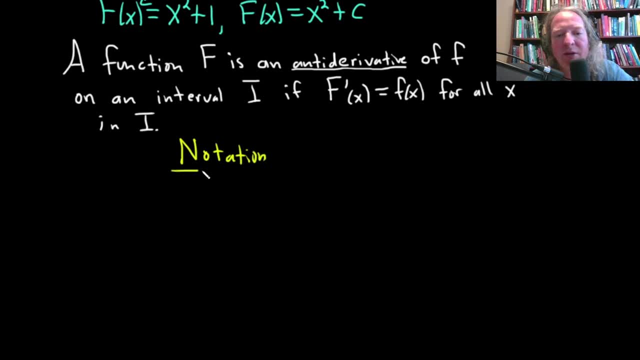 we're going to use. so the process of finding an antiderivative is called anti differentiation. right, we're going backwards. so instead of differentiating, we're anti differentiating, and here's the notation we use. so we have this elongated s symbol. this is called like the integral symbol, so it's the. 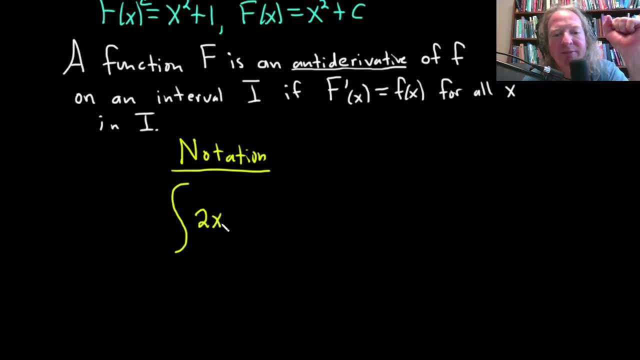 integral symbol. and here we have 2x and then we have DX, and we said that our best answer was this: one x squared plus C. so in this example which we did in our head, we looked at the 2x and we said: oh, what's a function whose derivative is 2x? we said: x squared. this is the notation. 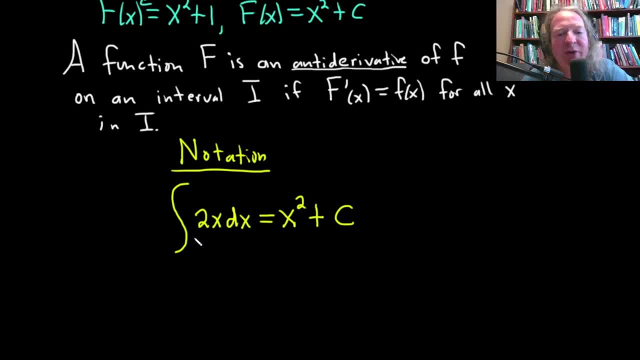 you would use. so this process of finding an antiderivative is called anti differentiation or integration. so this piece here has a name. this is called the integrand. it's really important to know this, because when you're talking to people about mathematics you say, well, my integrand you know I couldn't factor it. 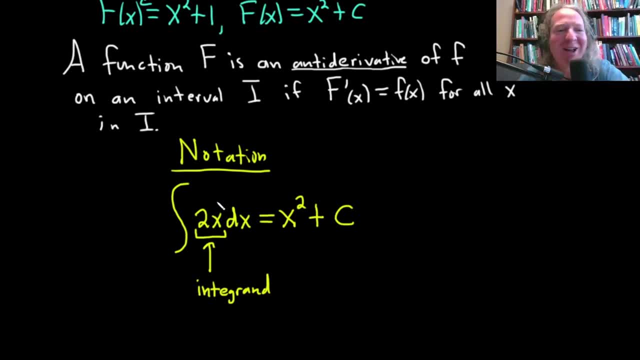 or you know you can talk about the integrand because, because you know what it is, this piece here, this DX, is a function that we can do with automatic. this tells you what variable you're integrating with respect to. so i'll just say variable of integration. so, because it's math, we have more than one variable. sometimes we integrate with respect. 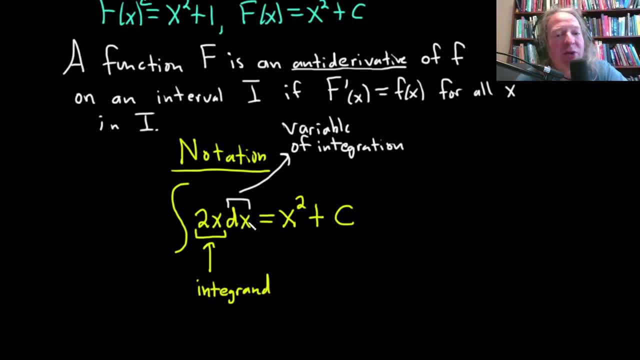 to y, in which case you would put a, d, y. sometimes you do theta, sometimes you do r. if you study multi-variable calculus you'll do x, y and z in the same problem. so you'll have dx, dy, dz. so it tells you the variable. so here the variable is x. this here is our anti-derivative x, squared in fact. 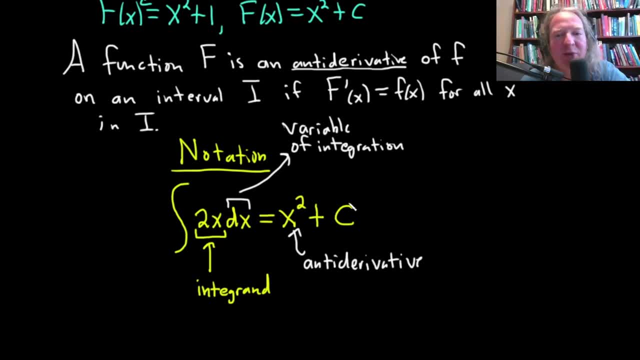 this whole thing is an anti-derivative. you could say x squared plus c is the anti-derivative, but i'm just going to single out x squared just so i can label this one as well. this one has a name. we called it an arbitrary constant, but it's actually called the constant of integration. 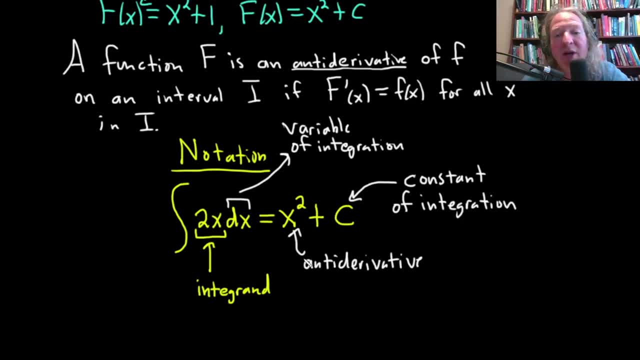 okay. it's the constant of integration. it's really important to include it. there's infinitely many solutions right. there's infinitely many choices for c. there's infinitely many anti-derivatives, really, really important to note. and this elongated s looks like someone took the letter s and stretched it. this is the integral. 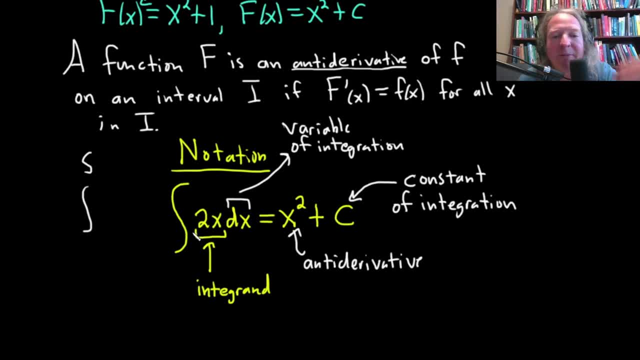 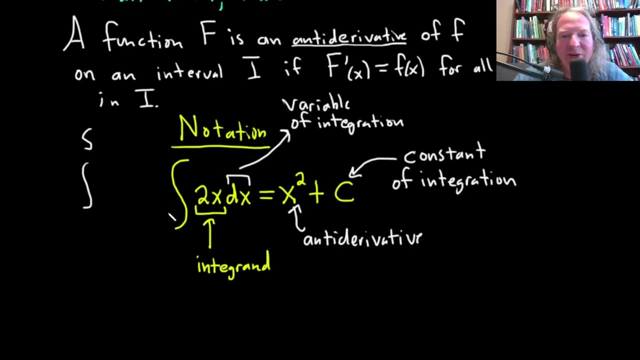 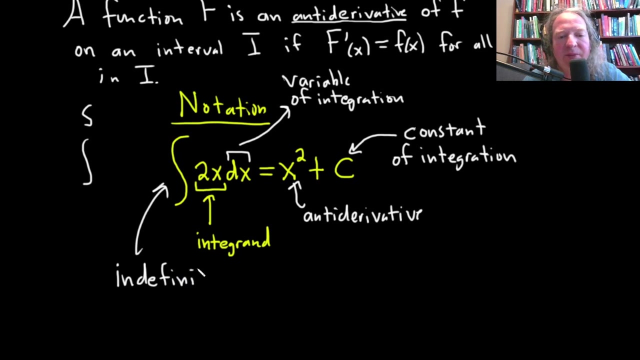 symbol. so again, this process of finding a function whose derivative is 2x, this process of going backwards, it's called anti-differentiation or integration. this is called an indefinite integral, so indefinite integral. i'm going to write that down. so this is an indefinite, in definite integral. a natural question then comes into play: what is a definite integral? 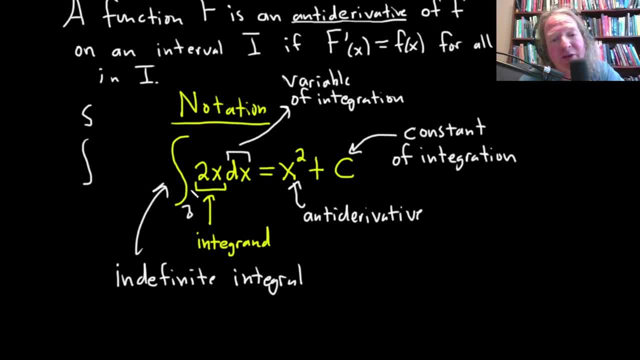 a definite integral is different. you're going to have like numbers here, like you might have a three here and a four here. that's called a definite integral. those are studied later. uh, you have to learn about riemann sums and some stuff like that, but for now we're going to stick. 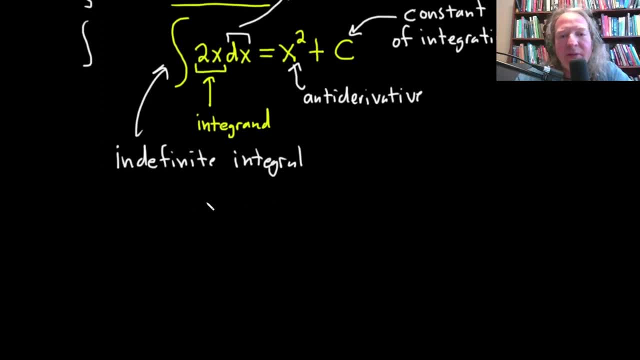 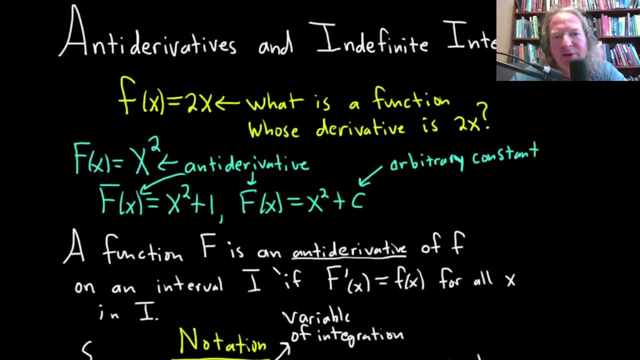 to the definition of a definite integral. so, in general, um, to do this it's pretty tough right, like we had to. you know, i picked this example for this video because it's easy, right, so i wanted to pick something that most people who know very, very basic calculus can do and understand. yeah, okay. 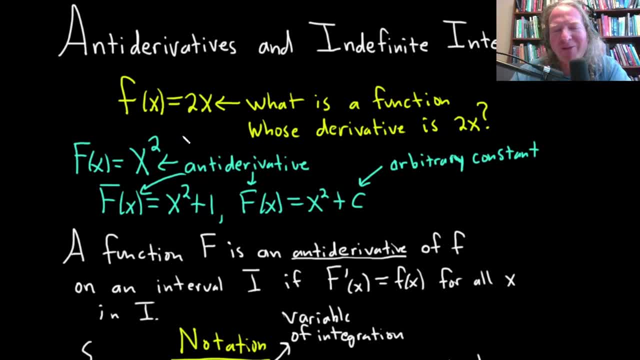 what's a function whose derivative is 2x, uh, x squared. but if i say, hey, what's a function whose derivative is, you know, x plus 1 over x cubed, plus 1 minus the secant of x, like you know what, what's that going to be? well, it's a little bit more difficult. 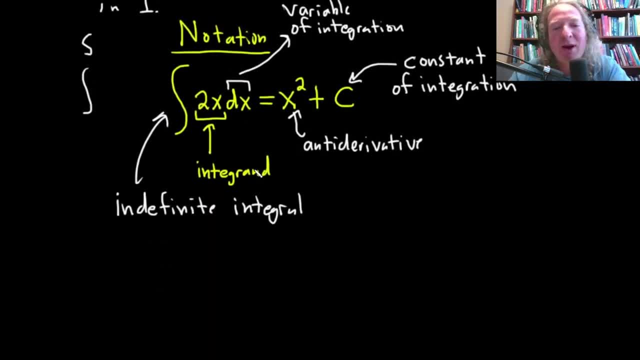 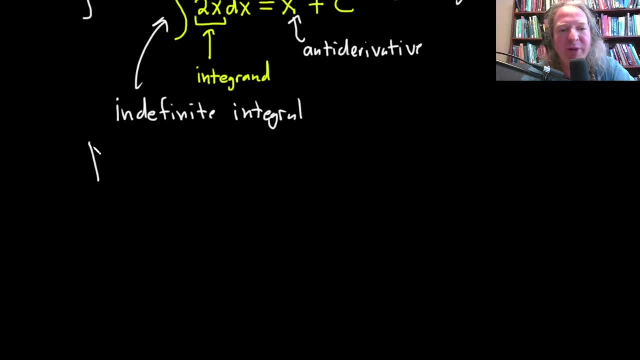 right. so you need formulas in order to do these problems. so now i'm going to give you a list of all of the basic formulas that you need for integration. so formulas, and we'll justify each one at least logically, and in some cases i'll be able to give you an example. in some cases, 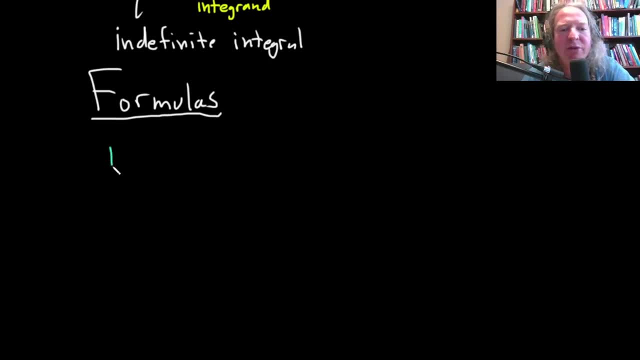 i really won't, not until until later. so the first formula we're going to look at is, if we're trying to integrate zero, okay, zero. we're looking for, uh, the anti-derivative of zero. we're trying to anti-differentiate zero- lots of ways to say similar things. so this integral we have. 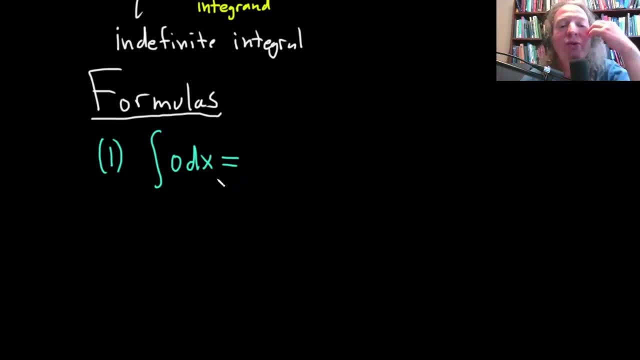 to integrate zero. so you ask: what's a function whose derivative um is zero? well, any constant function will work. let's just go with c, right? c will work because if you take the derivative of c, you're going to get zero. right, the derivative of a constant is zero, so that one's pretty easy. 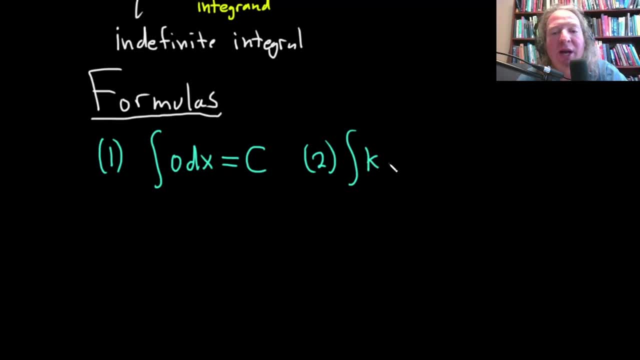 how about this one? let's say, we have a constant, which i'll call k, with respect to x. so the variable is x. what's a function whose derivative is x? well, it's going to be kx, and then, of course, plus our constant of integration, and you can always check your answer. 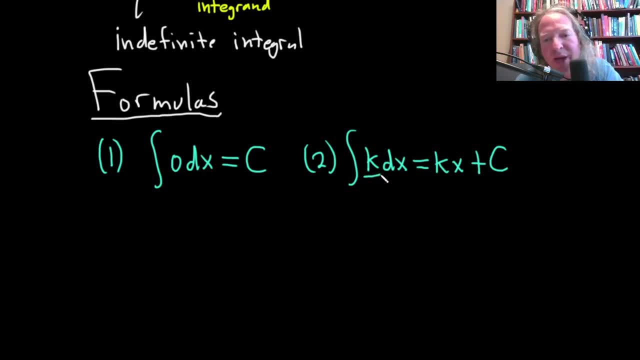 if you differentiate this, you should get the integrand see how important it was to know what it's called. get it out of the way helps to know. so the derivative of x is 1, so we just get k, and the derivative of c is 0, so it goes. 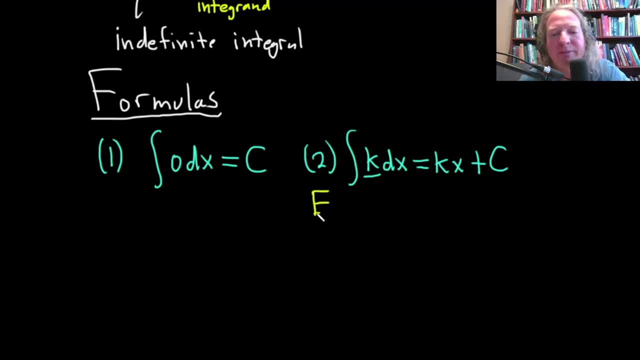 away. let's do an example with this one. we can do a simple one. let's say we want to integrate 2 with respect to x. so in this case, there's two ways to do it. method one: you ask yourself what's a function whose derivative is two? hmm, two x. and then don't forget the plus c. 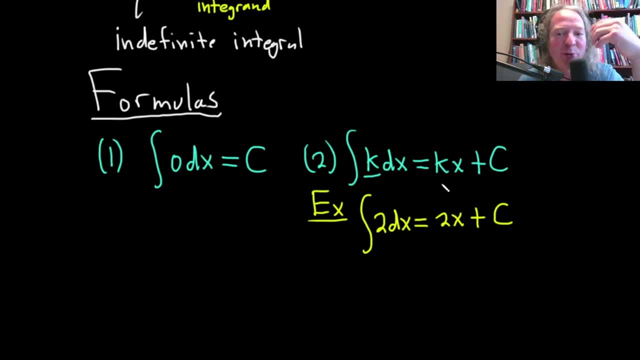 method two, which is the way i do it, which is much more mindless: uh, it requires less brain cells. you see the two, it's a constant by itself. you just put an x next to it, simple, right. doesn't matter how tired you are or how much math you've been doing if it's a number by itself, and it's with. 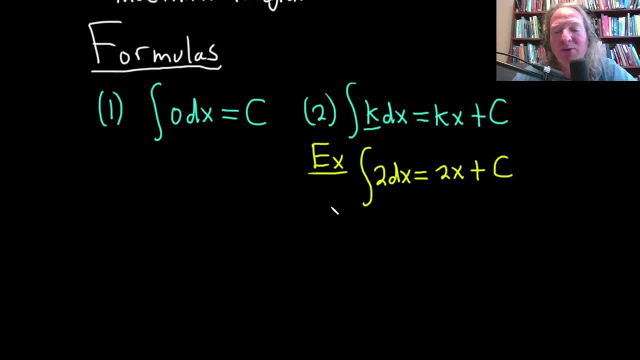 respect to x. you put an x actually. this leads me to a point. let's say, instead it was 3d theta. say what? what's going on, trig? yeah, i want to introduce a theta. why not, right? so in this case it's 3 theta plus c. so it depends on the variable. that's the purpose of this. it. 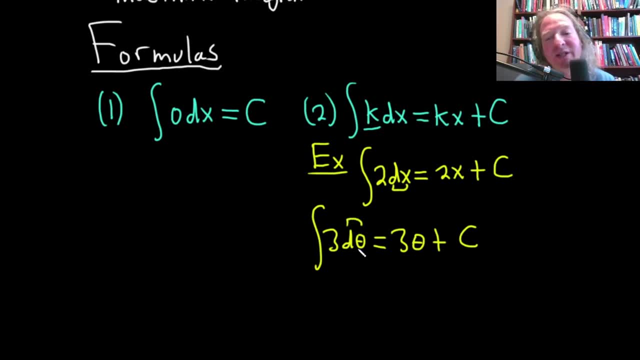 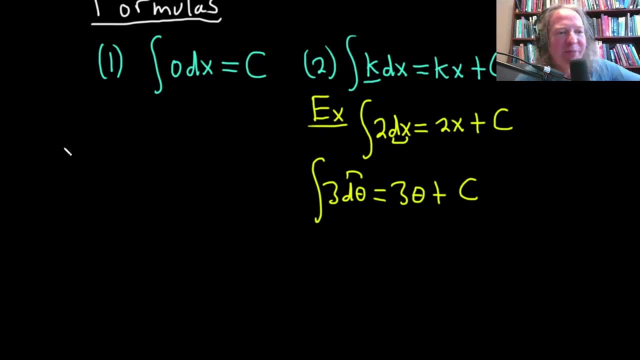 tells you what the variable of integration is. so in this case, it's d theta, so we put a theta. if it's dr, you put an r, etc. all right, let's go to our next formula, which i'm just doing these off the top of my head: um, how about this one? if you have a constant times, a function? 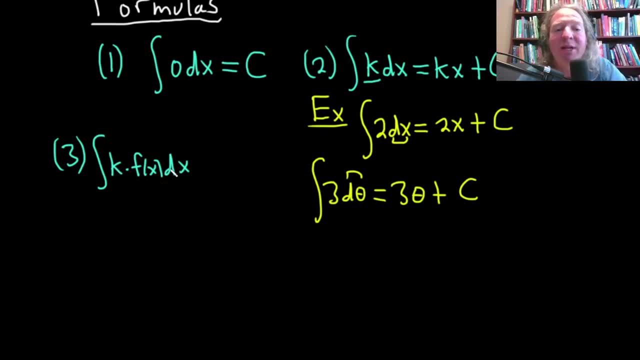 okay, you can pull the constant out because it doesn't depend on the variable x. so this is equal to k times f of x dx. this will come up sometimes later. just know that if you have a number you can, you can pull it out and and there's no issue. 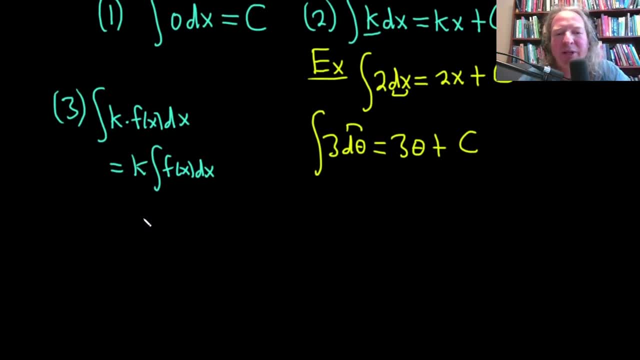 as a concrete example, i guess i could do one here. it's a little bit silly, but let's do it. let's say you're trying to integrate a five with respect to x. you're saying: huh, i don't really like the five, so i'm going to pull it out. so you pull it out and 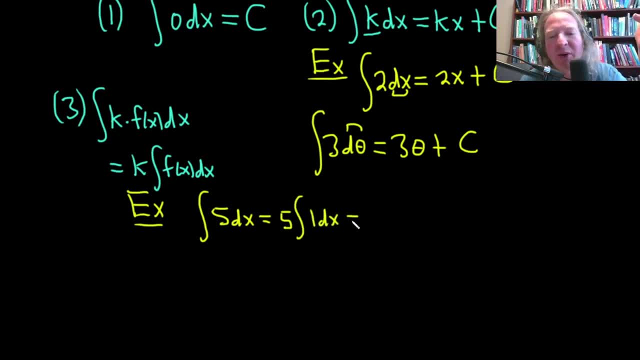 just left with one dx and you say: oh one, i can integrate one. that's just x, right, because one times x is x, the derivative of x is one, so the integral of x integral of one is x rather. so to integrate one, you just use this rule, right? so you just put an x next to it, so you just get 5x, let's. 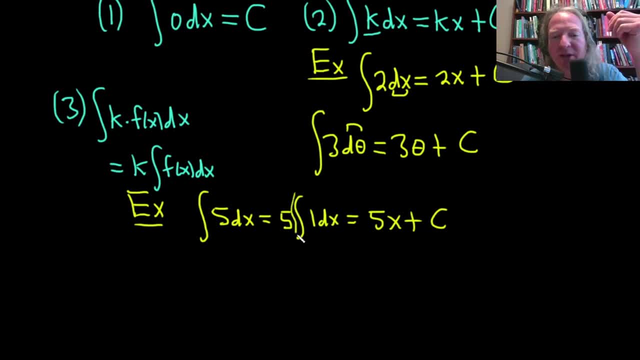 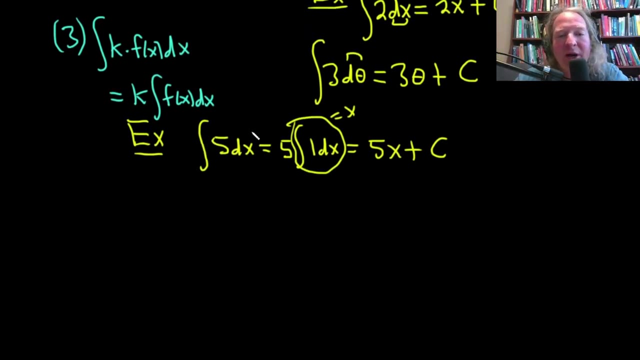 see. so a pretty useless move here, right? so you integrate this and you get x, and then you just multiply by five and you get your answer. so not very useful, uh, in this particular case, kind of a example. but the point is you can pull numbers out which can be useful sometimes, just not in this. 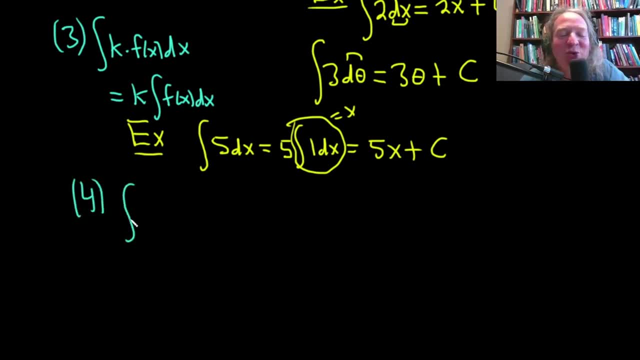 particular case here. this next rule is very useful. it says: if you have more than one term in your integrand you can separate it into two integrals. so if you have, say, f of x plus or minus g of x with respect to x, you can break this up into two separate integrals. we have the integral. 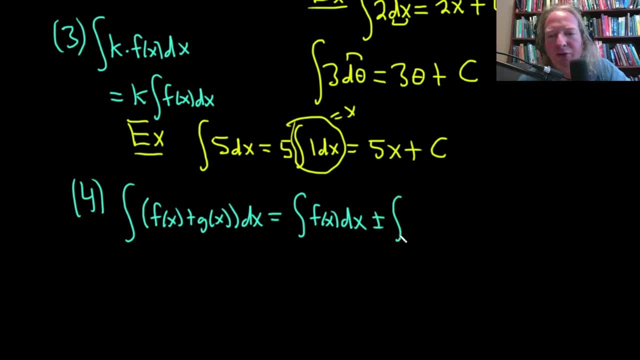 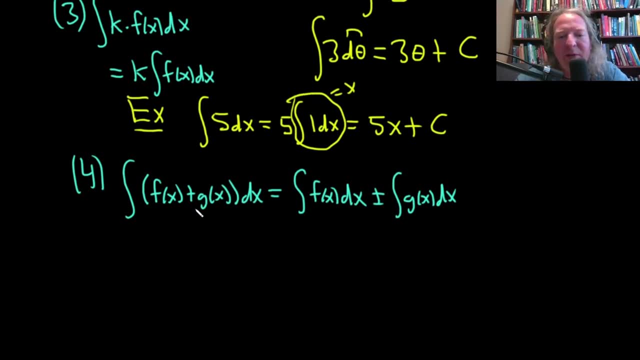 of f of x with respect to x, plus or minus, the integral of g of x with respect to x with respect to x. very useful and once we know more i could do an example of this. but basically it means you can integrate term by term. if you have five things you can. 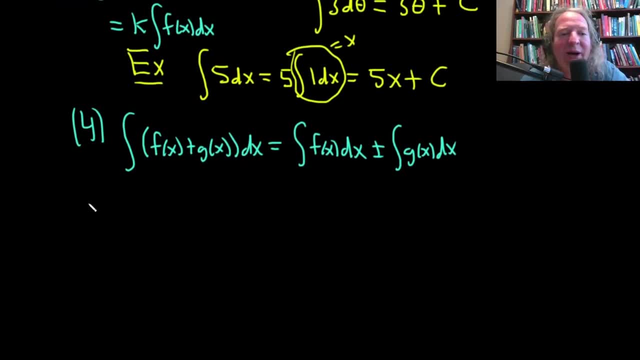 break it up into five integrals. that's okay as well. five, uh. this next one's really important. it's called the power rule. there's so many power rules in mathematics that it almost pains me to use the word, but it's okay. context is key. so this is the power rule for integration. 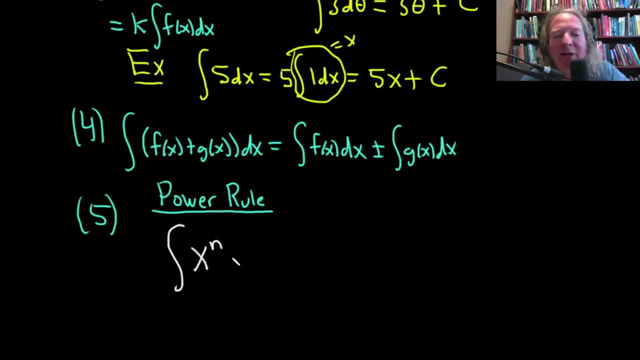 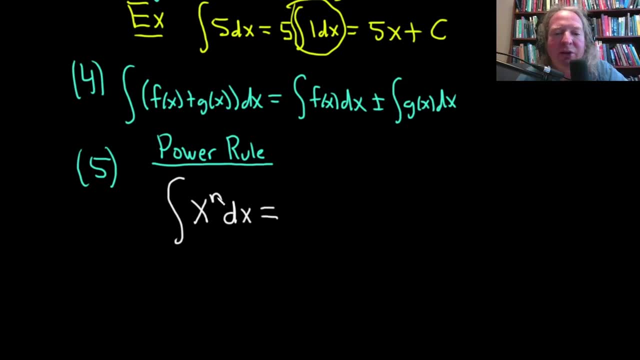 so if you have x to a power, say x to the n, and you're integrating this with respect to x. so what you can do is basically you just take the exponent and you add one, so this is x to the n plus one, and then you just divide by the one and then you add your constant of integration. 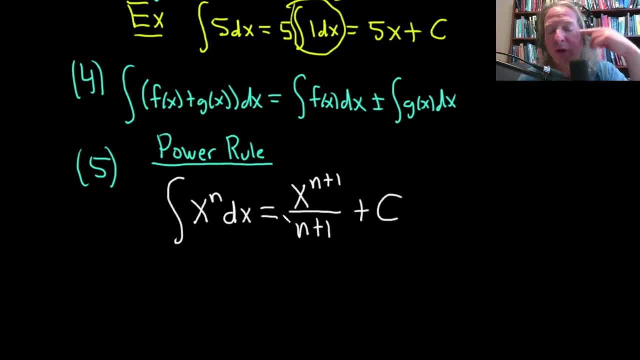 capital c. so very, very powerful rule. now, if you're thinking like- i don't want to say a person, but sometimes you get into the habit of thinking: when doesn't it work well, when doesn't this work well? if n is negative one, it doesn't work. so this is only valid for n not equal to. 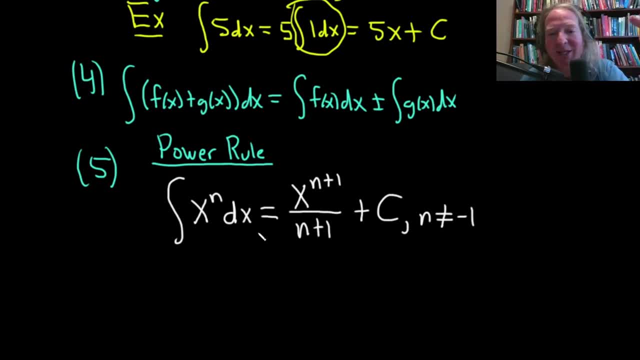 negative one, okay, and the natural question then to ask is: what do you do when n is negative one? i'll show you, and i'm going to put it in red up here, if you have x to the negative 1- this is later. this is going to be the natural log of the absolute value of x. 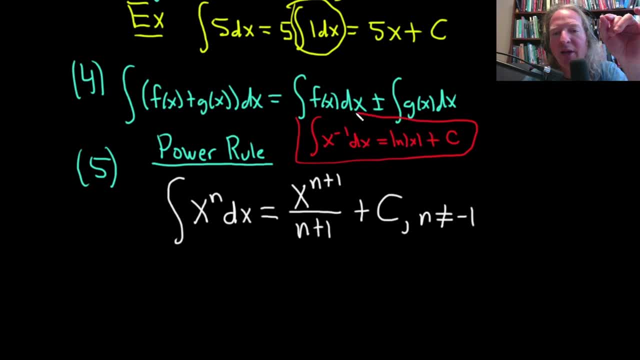 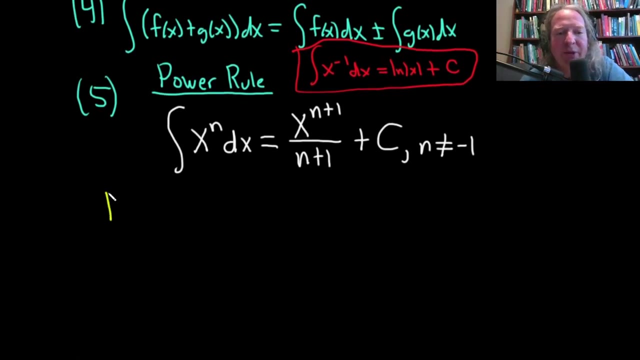 plus c and this. this is something you learn later in calculus. uh, we're not going to be discussing it in this video, it's it's taught much later. but for every other choice of n? um you can use this formula, so very powerful. let's do an example right away so you see it. so let's say we have to. 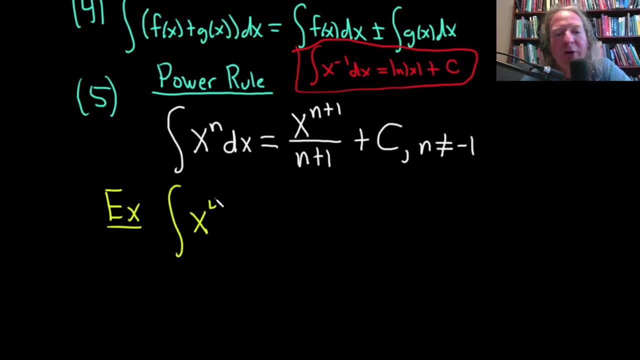 integrate x to the fourth with respect to x. so in this case a newcomer to study of calculus might say: hmm, okay, so the exponent here is 4.. this is the value of n. so if i'm going to apply this formula, it's x to the 4 plus 1 over 4 plus 1. 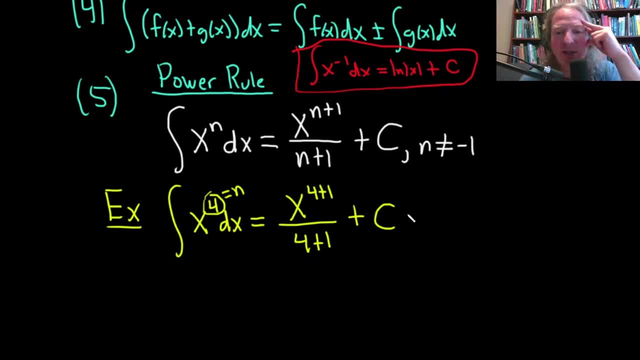 plus c, and that would be 100, correct. and so this is equal to x, to the 5 over 5 plus c. so this would be the answer now. in general, you do want to eventually move past the n-th value, this type of computation. you want to eventually skip this work because it really clutters your 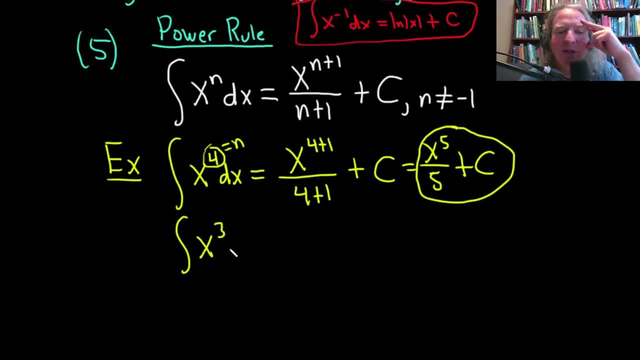 problem. So when you see a problem like this- let's just say x cubed dx- you basically jump to the solution: 3 plus 1 is 4, and then you just divide by the 4, like that plus c. So you want to. 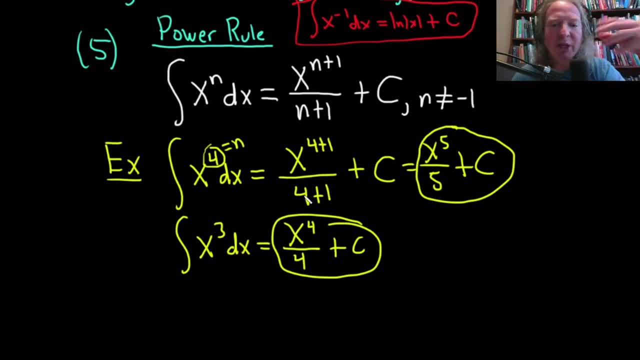 skip this middle step. It's not wrong, it's just it really like slows you down and it's just the math gets really long and involved. So anytime you can skip a step that's very, very easy to do mentally like this, it's recommended that you do, And this just doesn't look pretty when you have 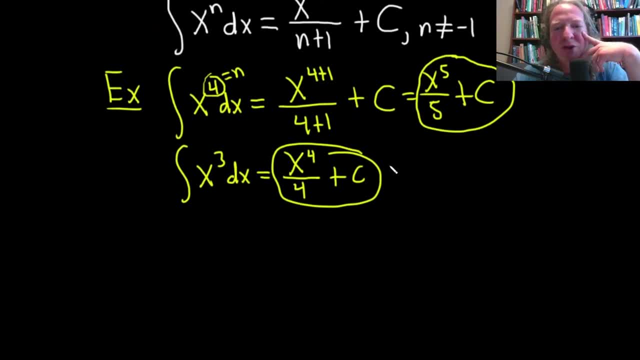 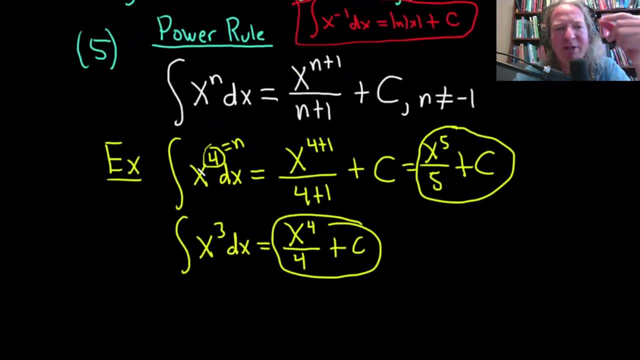 six of these in the same problem, you know, so worth just going to the answer. So very, very powerful formula. Okay, I think what's left now are the trig functions. I guess I've been numbering these, so I'll call this one 6. And the trig functions often intimidate people because 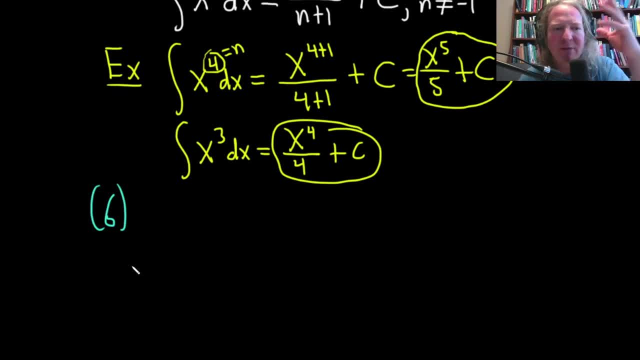 people see these formulas and they think, oh wow, I'm supposed to memorize all of these. You are, but at the same time you can think about them a little bit differently. So I'm going to show you how I think about these and maybe 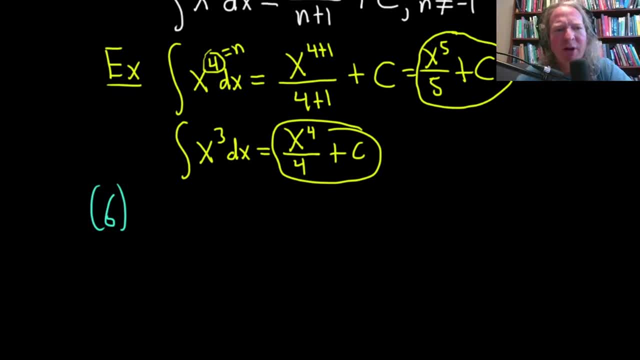 that will work for you. So let me just switch colors here. For some reason, my pen got really thick. I had to. I can control how thick my writing is. Watch this. I can write really thick or I can write really thin. I'm just trying to find a happy ground here. Here we go, let's try. 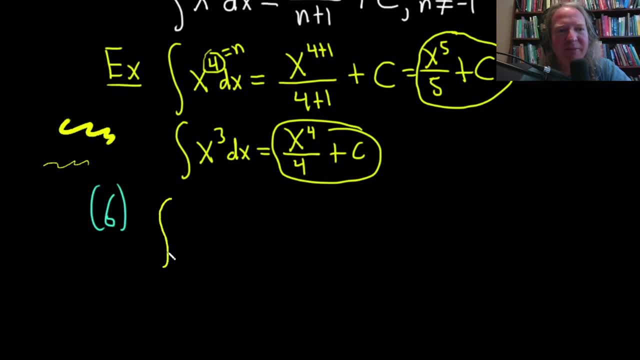 this one. So let's try to integrate. that's pretty good. Oh, I'm using graffiti pen. There we go. let's go back to pen. Let's try cosine x. There we go Back to regular writing, The integral of cosine x. So when you're trying, 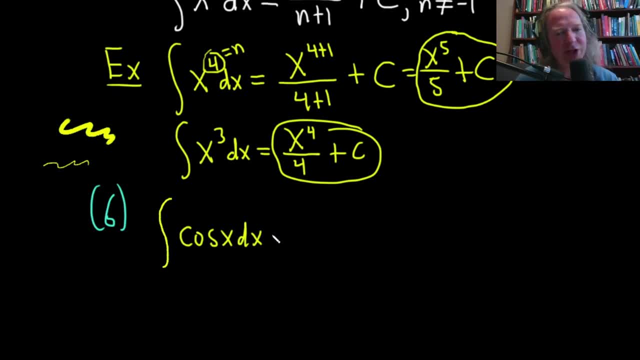 to integrate cosine, you're asking yourself what is a function whose derivative is cosine Sine? This is sine x, but that's not it. We still need a plus c, So pretty easy. So whenever you look at the integral of cosine, 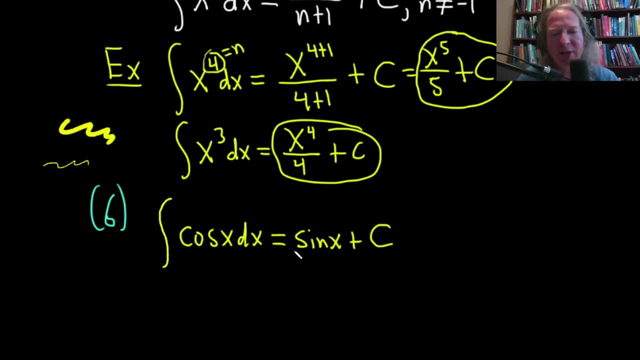 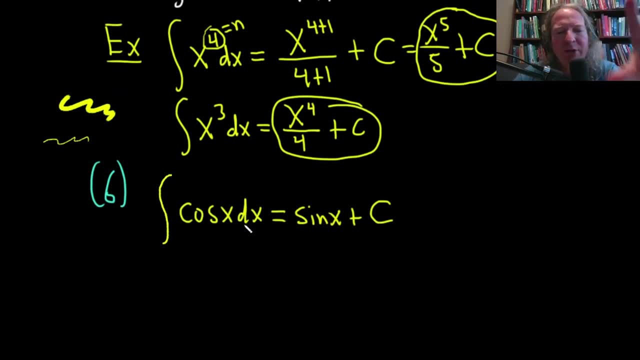 if you don't have it memorized, you can memorize it. You can say, hey, the integral of cosine is sine, But maybe there's just you're just having a hard time finding room in your brain to memorize it and you're just refusing to memorize things, which I have a habit of doing. I like to know how. 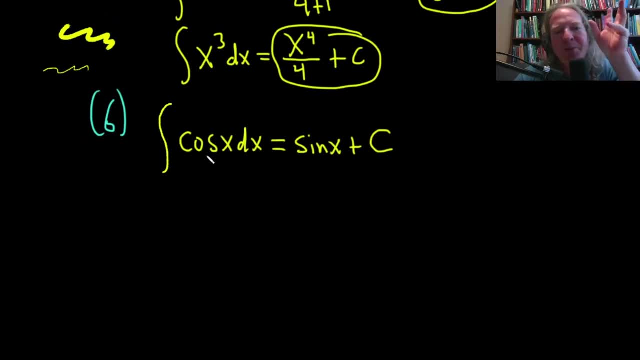 things are derived and it's just a habit. So you're trying to integrate cosine. you say, oh, I forgot what that was. Oh, but wait, what's a function whose derivative is cosine, Oh sine, The derivative of sine is cosine. Yep checks You. differentiate this. you should get your. 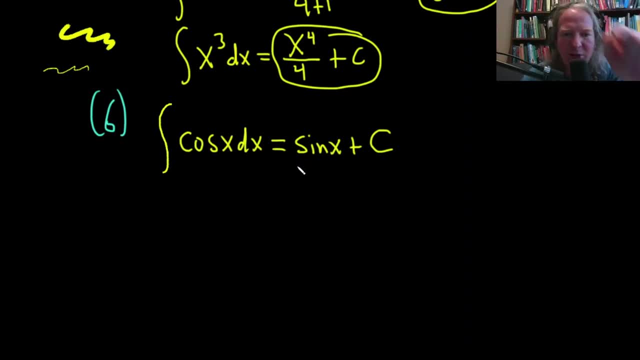 brand and it certainly works, because the derivative of sine is cosine. What about this one? There's a reason: I did cosine first, because it's easier. This one's harder. So what's a function whose derivative is going to be sine? Well, the derivative of cosine is negative sine. 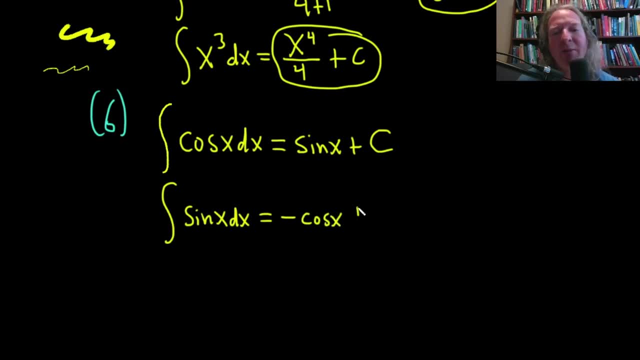 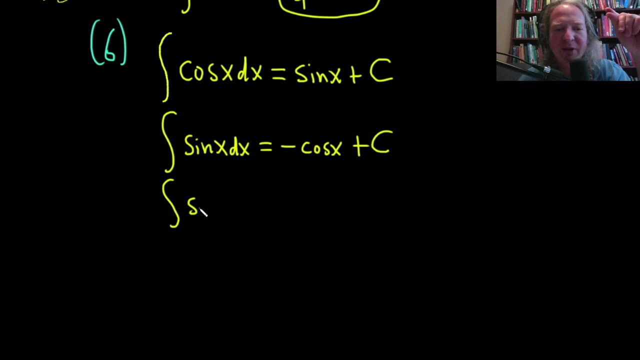 So this is going to be negative. cosine x and then plus our constant, And you can check right. The derivative of cosine is negative, sine. We've already got a negative here, so negative and negative is positive. so life is good. How about this one here? Secant x, tangent x, These. 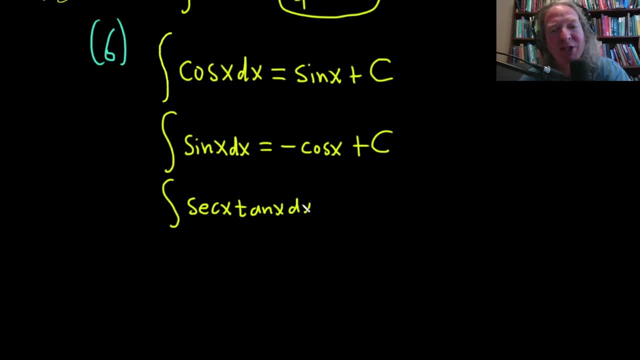 are strategically picked. by the way, You might say: what about secant? Why'd you jump to secant? tangent Secant is a whole other story. right, Integration is not as easy as differentiation. The integral of secant requires other techniques which we'll learn later. So you have secant times. 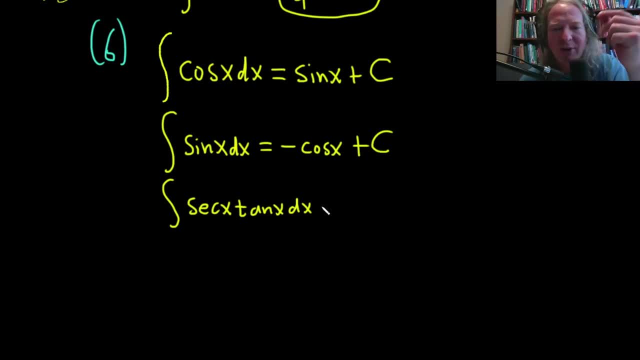 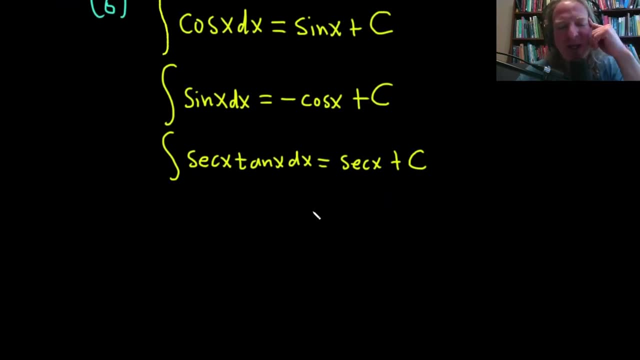 tangent. What's a function whose derivative is secant tangent? Well, secant, This is the secant of x plus our constant of integration, capital C. And how about secant squared? That's another one we can do now. Secant squared x- dx. So what's a? 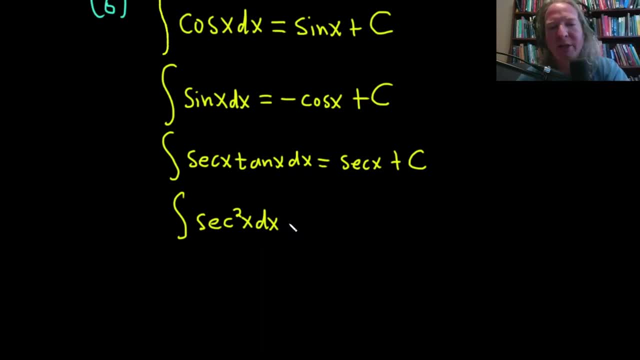 function whose derivative is secant squared. Well, that's just going to be tangent x plus C, right? Because the derivative of tangent is secant squared. And then we get to the unpopular ones, the ones that don't come up. So we're going to get to the unpopular ones, the ones that don't come up. So much Cosecant x, cotangent x, dx. So what's a function whose derivative is cosecant cotangent? Well, the derivative of cosecant is negative, cosecant cotangent. So this requires a negative cosecant x plus C. Again, the derivative of cosecant is negative. 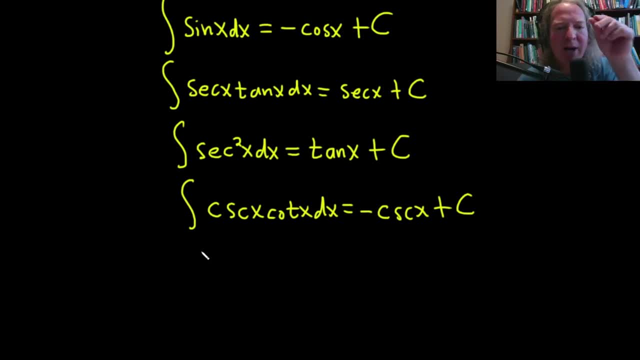 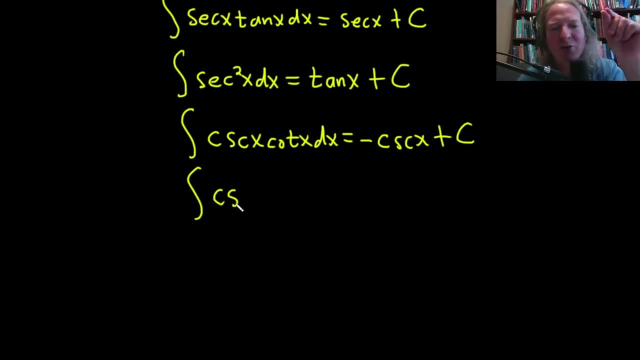 cosecant cotangent. We've already got a negative, so it will become positive. And the last one we're going to discuss in this video, the last formula- I know it's a lot of formulas- is cosecant squared x, dx, And in this case you ask yourself what's a function whose derivative is cosecant squared? 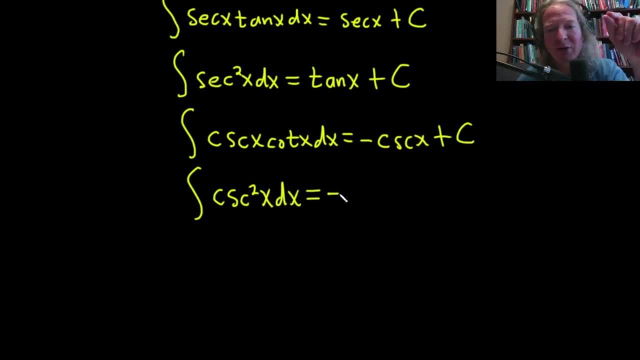 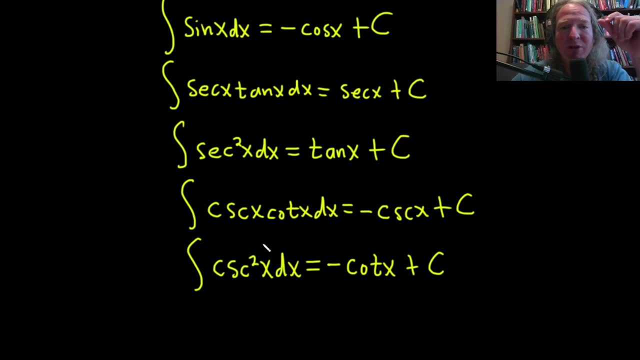 Well, the derivative of cotangent is negative cosecant squared. So this is going to be negative cotangent of x plus our constant of integration capital C. So wow, that's a lot of formulas And usually when people first see this they're like OMG, how am I ever going to? 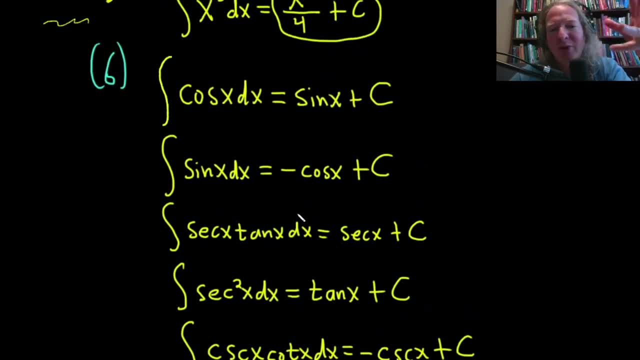 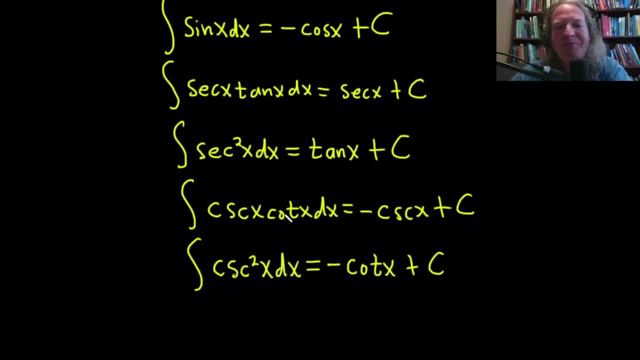 know this, But how did I just go over it? right, It's just all derivatives, So it's really the derivatives that give you the integrals, And at least for me that seems to work better. It stays in my long-term memory, It just works. 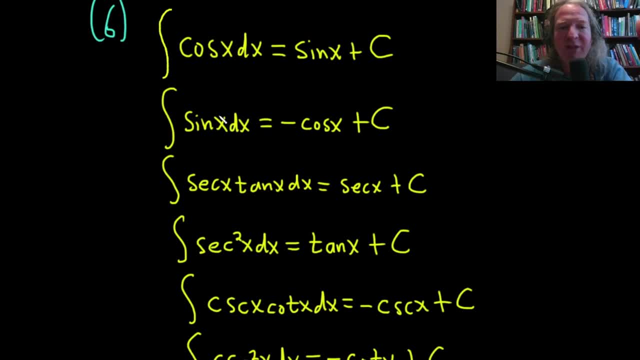 better because you know you integrate other stuff besides these things. You know you might have to integrate sine to the fourth power someday. That requires trig identities, requires a lot of knowledge. So I just feel like the less you memorize sometimes the better. And thinking, 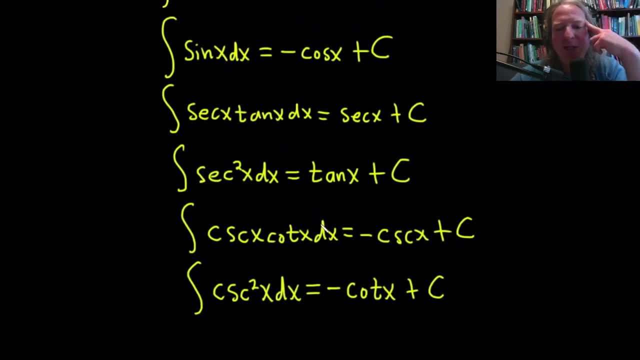 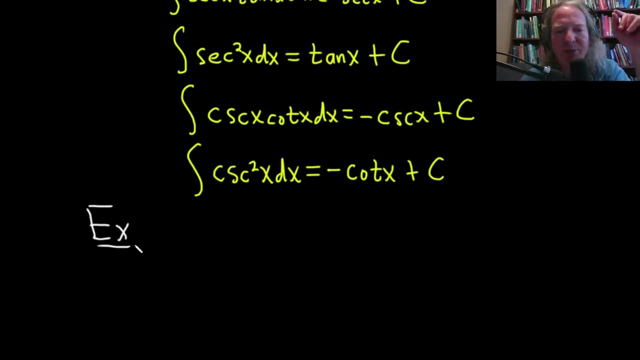 about it in terms of differentiation makes it a little bit easier. But I can do an example. I'm going to switch back to white And let's just do a simple example here. Let's say we have x to the negative four- Maybe not so simple- Plus five, plus sine x, dx. so now we have three terms, three terms. 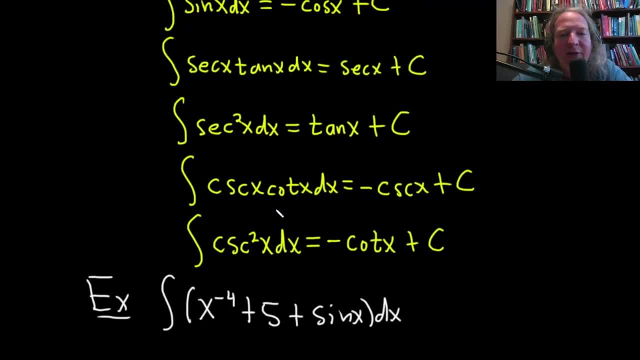 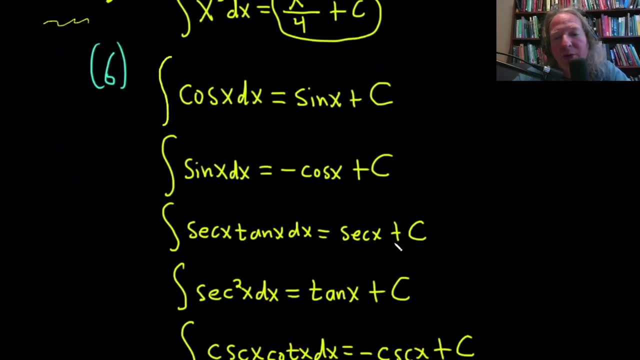 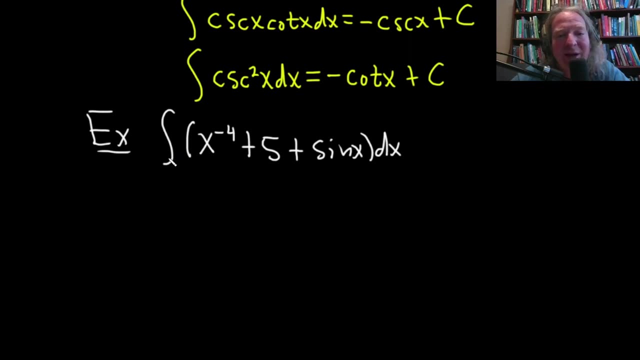 So we saw earlier that one of the rules said: if we have two terms, we can break it up into two pieces, but if you have three, you can do it also, you can break it up into three. the rule can be easily generalized, generalized to any finite number of terms inside the 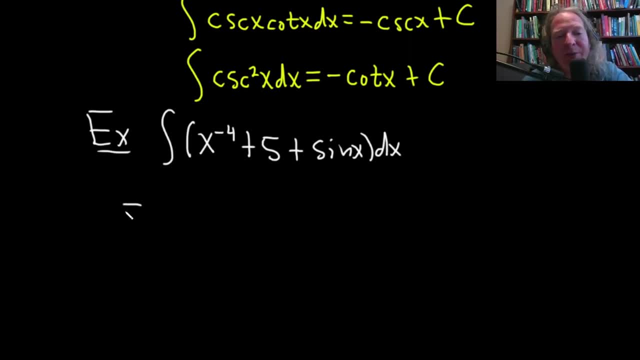 integrand alright, so let's just jump into it. by the way, when you integrate, you drop the integral sign and you drop the DX. okay, so? so we're going straight to the answer here. so here we have X to the negative 4, so we can apply the power. 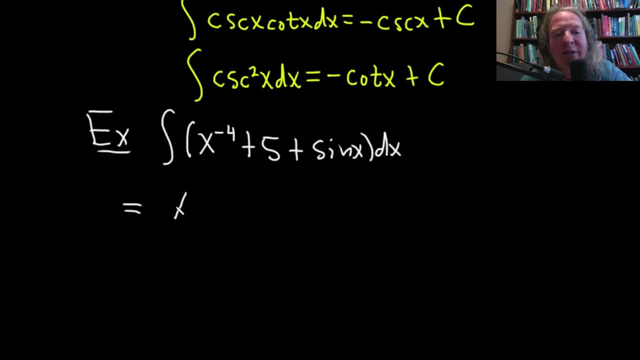 rule. so we'll add 1 to that, so it'll be X negative 4 plus 1 is negative 3, and then you divide by the negative 3. okay, plus you have a number by itself. just tack on an X trig function. hmm, what's a function whose derivative is sine? well, the. 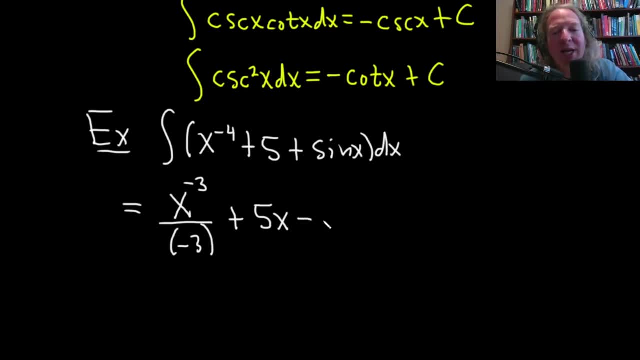 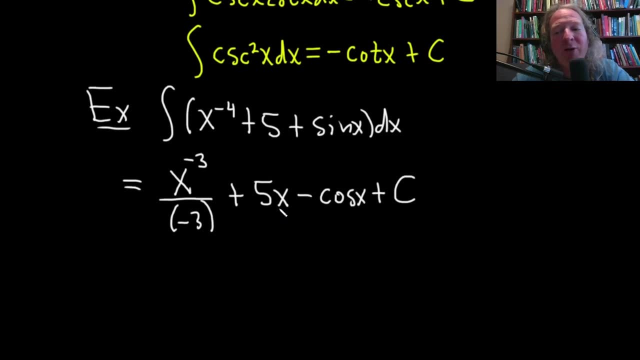 derivative of cosine is negative sine. so this is going to be negative cosine X, negative cosine X and then plus our constant of integration, capital C. it's not good form to leave your answer like this. so the negative on the bottom looks bad. I'm gonna write it like this: negative 1, 3rd times X to the negative: 3 plus 5x minus. 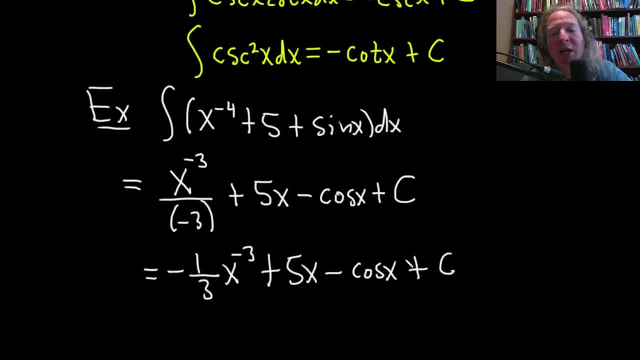 cosine X plus C, and that would be an acceptable final answer. some people ask about whether or not you should bring the this down, like you get this piece here and write it like this: negative 1, 3rd, 1 over X cubed. I think it doesn't matter. different people do it different ways. 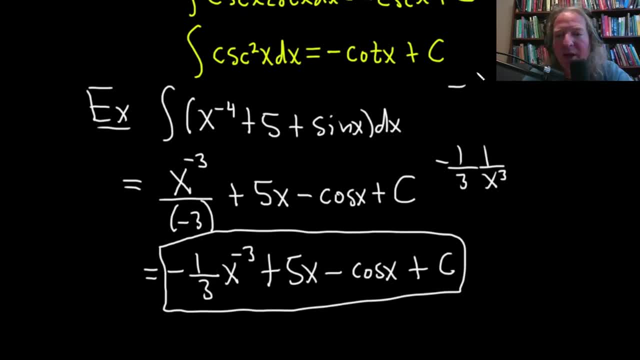 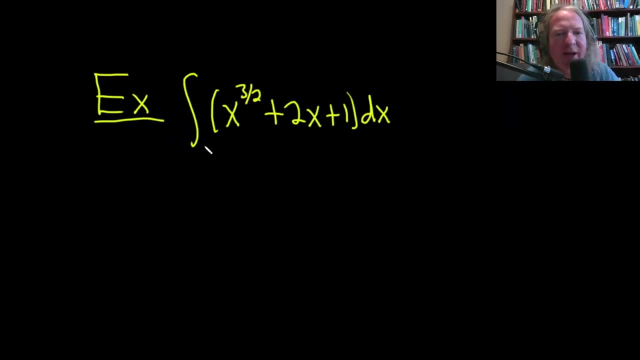 I've seen solutions in the back of books. they do it this way, they do it this way. some people will do this, which I really don't like. that's just more work. I personally prefer to leave it like this. so that is a simple example of indefinite integration. okay, let's do this example. here we have the integral of 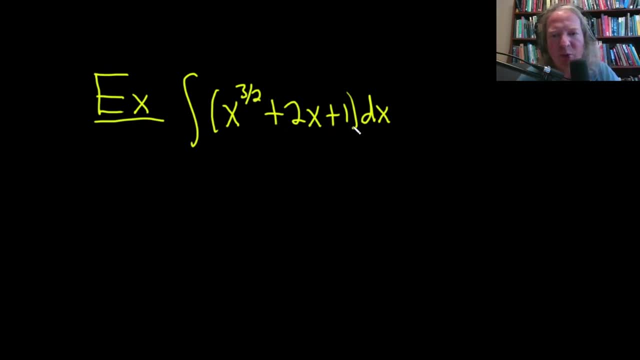 X to the 3 halves plus 2x plus 1, and again the DX here tells us what the variable of integration is. so solution: So in this case we can go ahead and just jump into it and use the formulas. So we're going to go straight to the integration. So here we can use the power rule. We actually have a 3 halves and 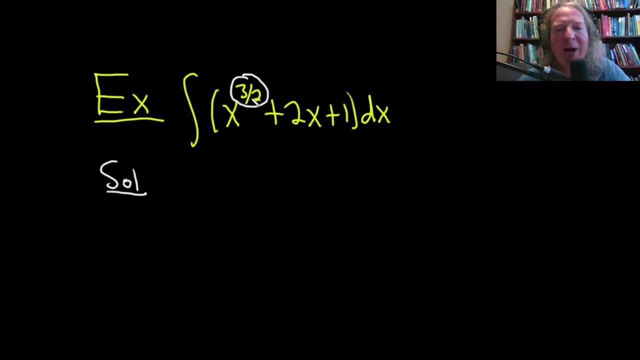 Remember the power rule says that whenever you have X to a power, as long as that power is not negative 1, You're basically adding 1 here to the exponent, So 3 halves plus 1. you come over here and write it: 3 halves plus 1. 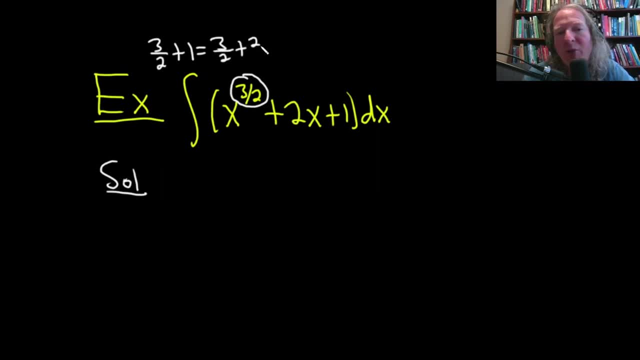 That's the same thing as 3 halves plus 2 halves, and I'm writing it that way so that we can actually, You know, perform the addition: 3 plus 2 is 5, so you get 5 halves. So what you would do is you would write X. 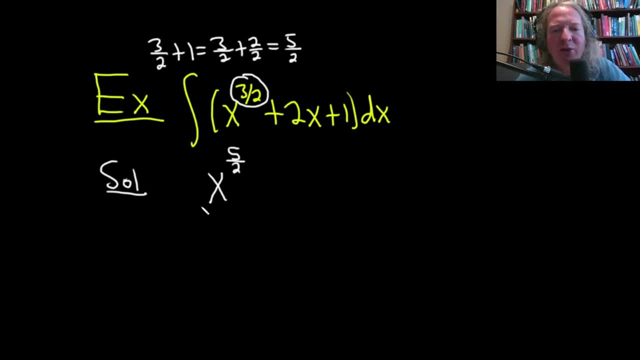 the 5 halves, And then you would divide and then You put the 5 halves down here. Okay, plus Same thing. here We have a number. Remember, when you have a number in front of an X, It just hangs out. So 2: 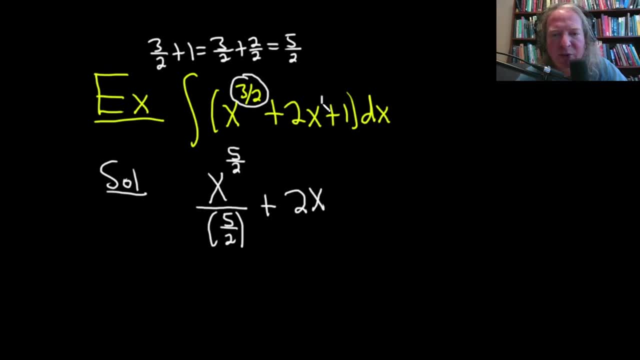 and we have X. the exponent here is 1, so 1 plus 1 is 2, and Again we divide by the 2. again the power rule, right, You add 1 and divide, add 1 and divide. so we added 1 to 3 halves. 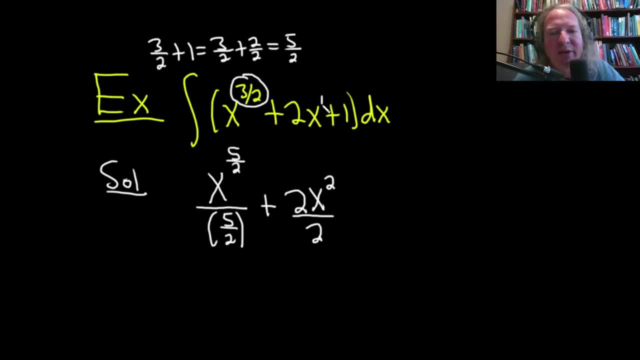 We got 5 halves we divided by 5 halves. added 1 to the 1, We got 2 we divided by 2. whenever you have a number by itself, Remember just tack on the X. So 1 times X is just X, Not correct? We're still missing the plus C. 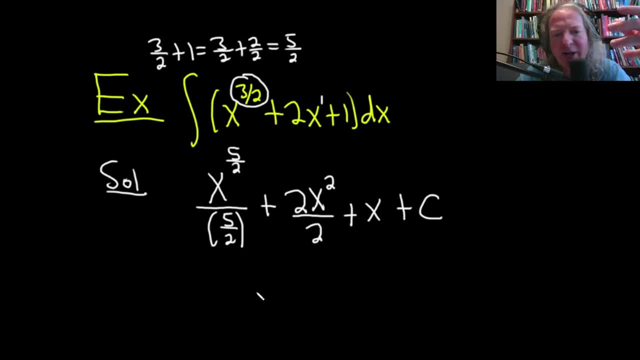 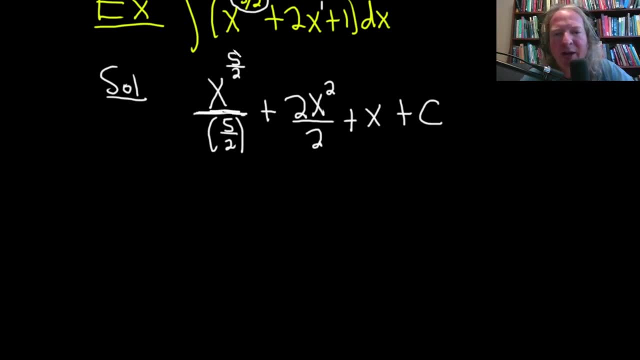 Typically, you don't want to leave your answer like this. right? It's not simplified and you have a complex fraction here, So let's clean it up. What's happening here is a division problem. we have this divided by 5 halves. when you divide, you really multiply by the reciprocal. 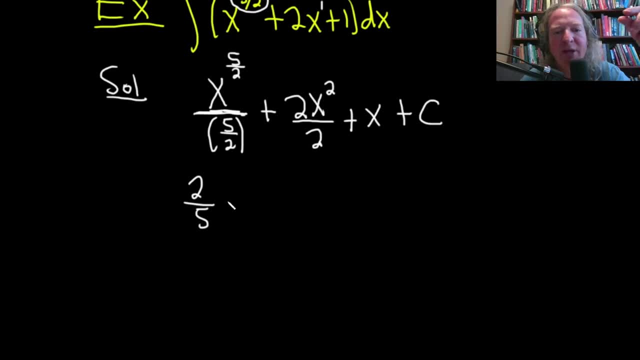 So this is really 2 fifths times X to the 5 halves Boom, this goes away. plus x, squared Plus X, and then plus our constant of integration, capital C, and that would be an acceptable Final answer in this example here. So super, super key. So again just adding, adding one here: 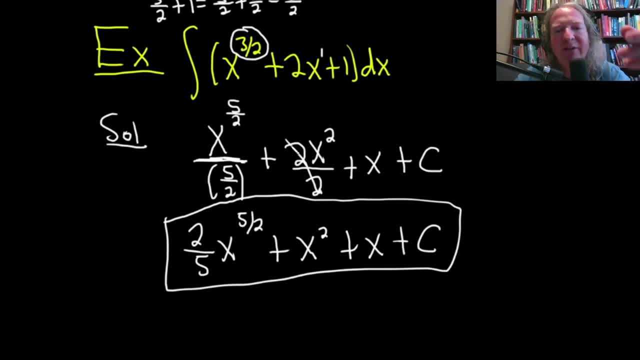 so two halves plus three halves is five halves Divide by five halves. One plus one is two Divide by two. You have a constant by itself. You just tack on the x and then you have a plus c pro. and then these: 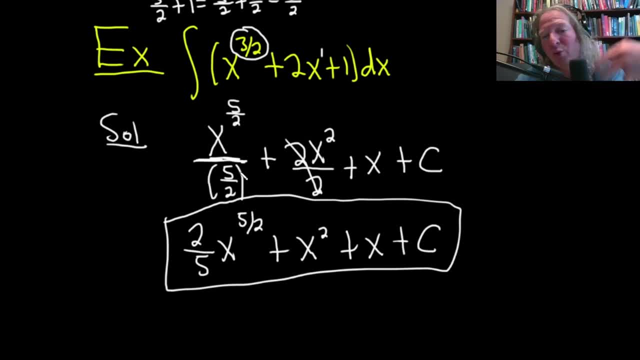 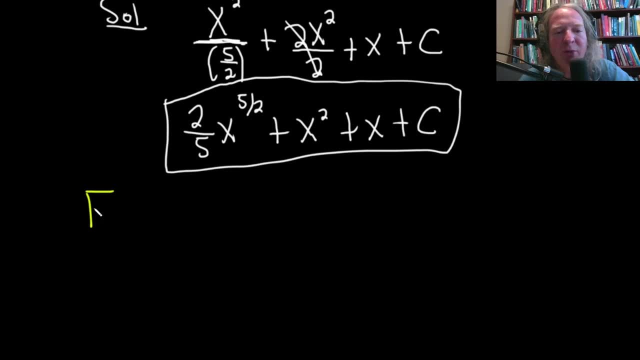 cancel. This is a division problem. When you divide by five halves, you're really multiplying by the reciprocal. Let's do another one. The best way to get good at integration is just to do a bunch of integrals. I mean, there's no better way to get good at it. I want to emphasize a point. 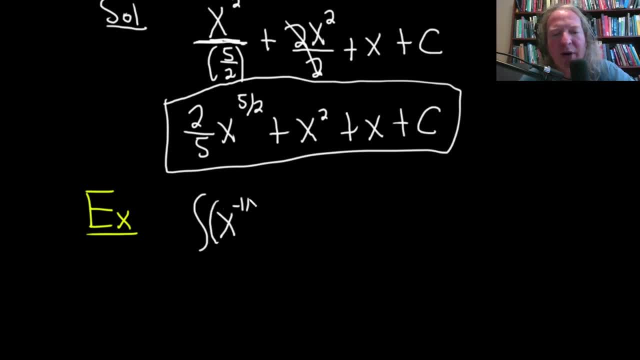 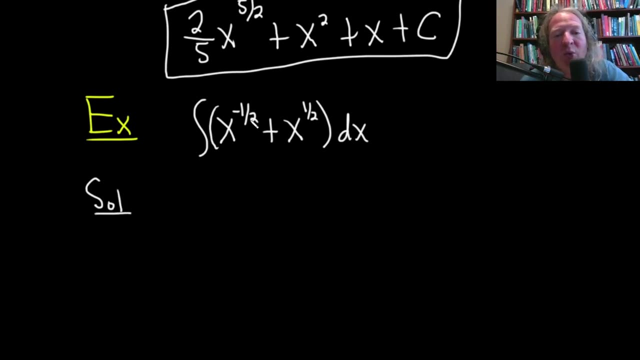 about fractions. so I'm going to do this. This is negative one half plus one half. dx. Let's make one up Here. we can use the power rule twice. Let's go ahead and do it. Solution: We're going to add one to negative one half. That's going to be negative one half plus one, which is really. 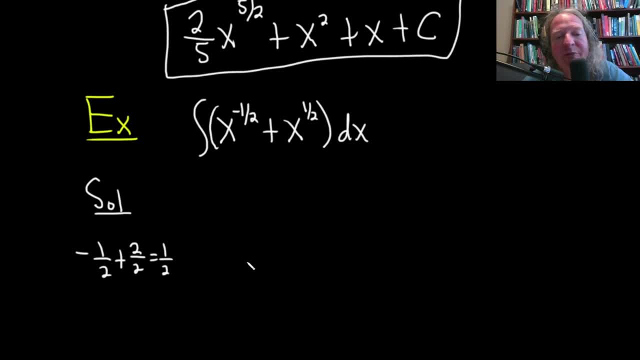 negative: one half plus two halves, which is one half, It'll be x to the one half divided by one half plus same thing. here We have a one half, We're adding one. It's one half plus two halves, which is three halves. It's x to the three halves. 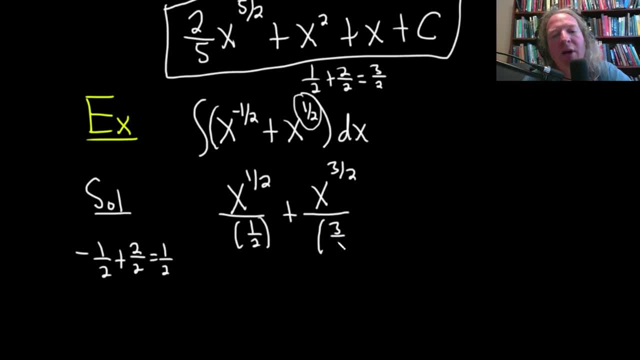 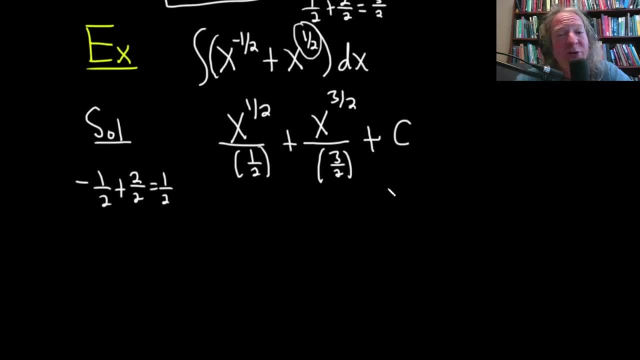 divided by three halves. and then we have our constant of integration, capital C. Then again we have these two halves. We're going to do a bunch of integrals, Two division problems. Whenever you divide, you multiply by the reciprocal Dividing by one half. 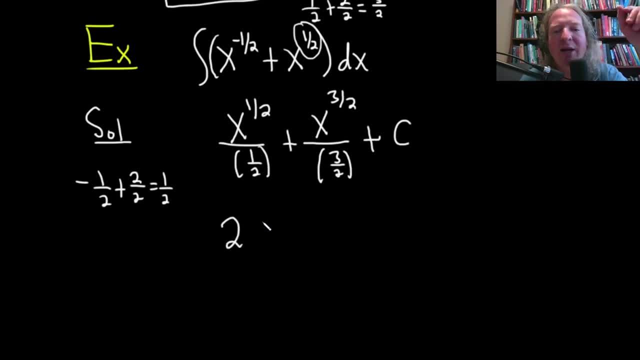 is the same thing as multiplying by two. This will be two x to the one half, which you can write as the square root of x, It's up to you. Plus. and then dividing by three halves is the same thing as multiplying by two thirds. This is two thirds x to the three halves plus C. That would be an. 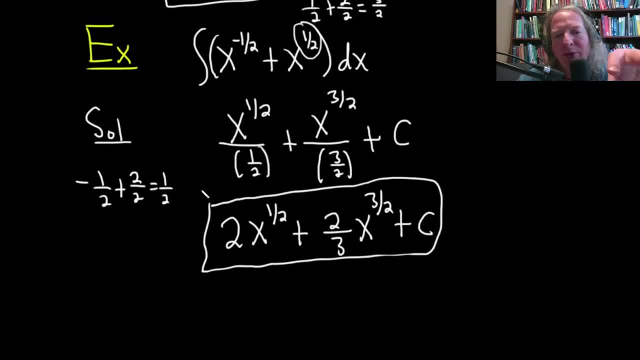 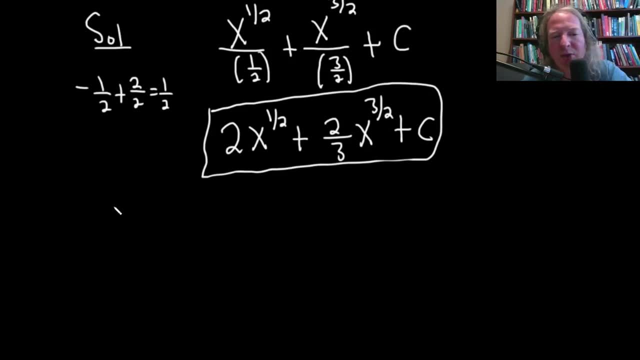 acceptable answer. Now, this is not how I would do the problem. I'm just doing it this way to show you. Let me show you what I would do when we're faced with a situation like this. I would take a shortcut. Let's say we: 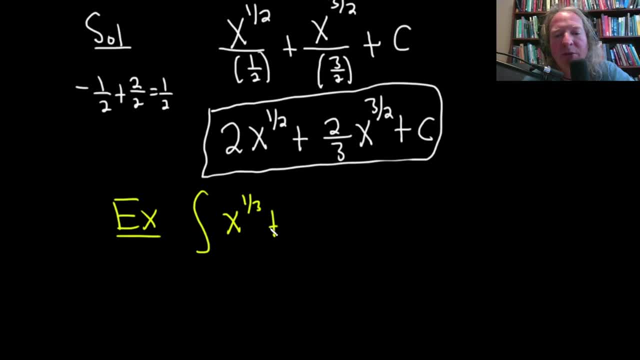 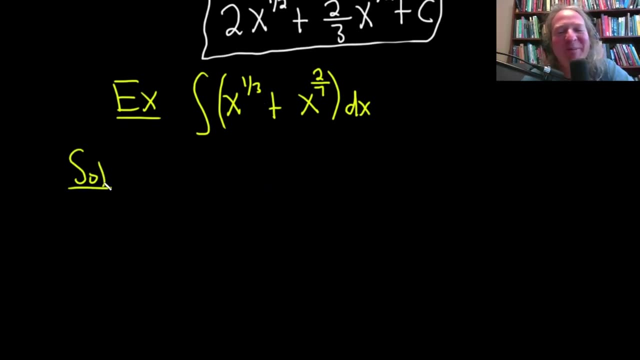 have x to the one third plus x to the two sevenths dx. Just dealing with these really bad fractions that no one wants to deal with, Let's do it. Solution: So we're adding one, right? We're adding one and dividing. We're using that power rule. So 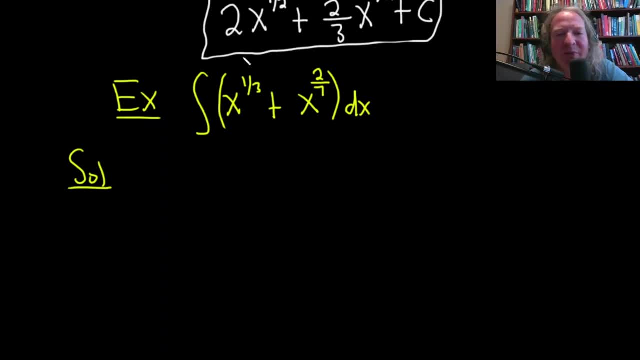 we have x to the one third, and then here we have x to the two sevenths, So here it's one third plus one, So think of it as a number over three. So one third plus three thirds, So four thirds. 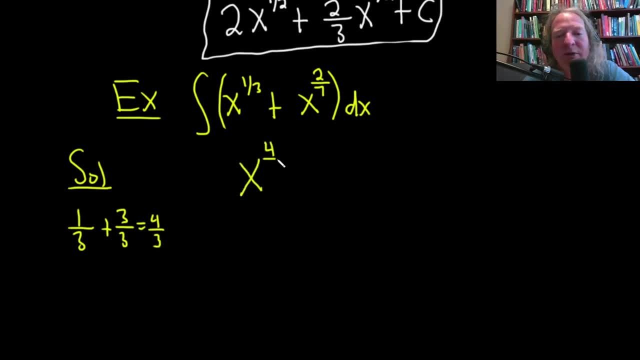 So it'll be x to the four thirds, okay, And we're dividing by four thirds. But when you divide by four thirds, you're really multiplying by three fourths. So we're dividing by four thirds, Boom. So you skip that step. So whenever you divide by a fraction, you can automatically turn. 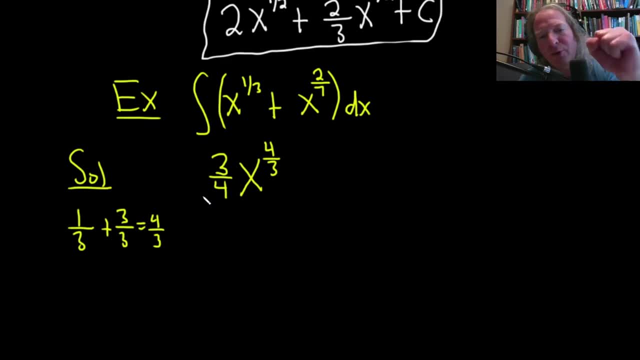 it into multiplication by the reciprocal, Super, super powerful right, So powerful It saves you so much time. So again, we add one to the one third, which is four thirds. We divide by four thirds, But instead of dividing by four thirds, since it's going to require cleanup anyways. 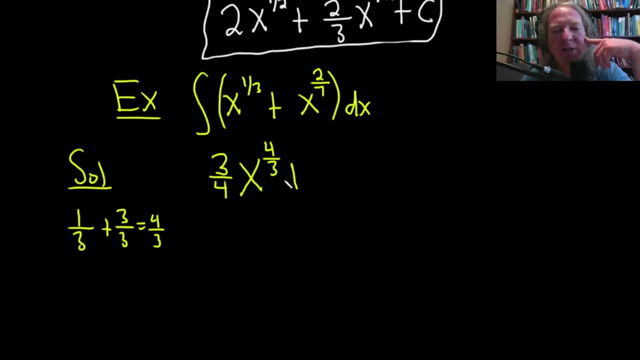 just multiply by the reciprocal Same thing here, Plus, we have two sevenths plus one. So think of one as a number over seven, which is seven sevenths, So it's going to be nine sevenths. So this will be x to the nine sevenths divided by nine sevenths, So it'll be: 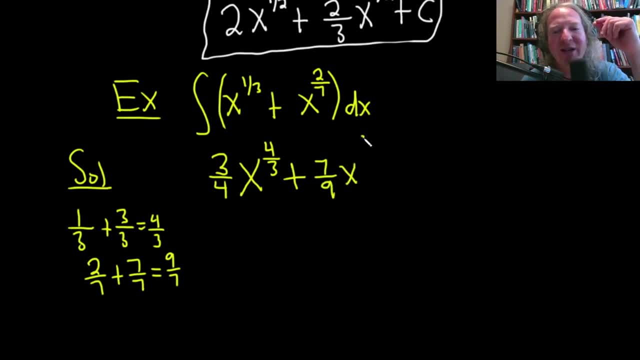 seven ninths times x to the nine sevenths. Again, it's x to the nine sevenths. Then you divide by nine sevenths, but you're really multiplying by the reciprocal, which is seven ninths. But that's not it. We're still missing something. 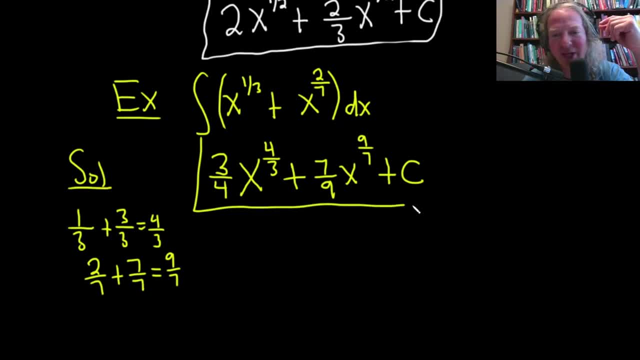 Super important. It's the plus c, So yeah, So whether or not you're comfortable skipping this step is up to you. It's a personal choice. If you want to show it every time, that's fine, right We? 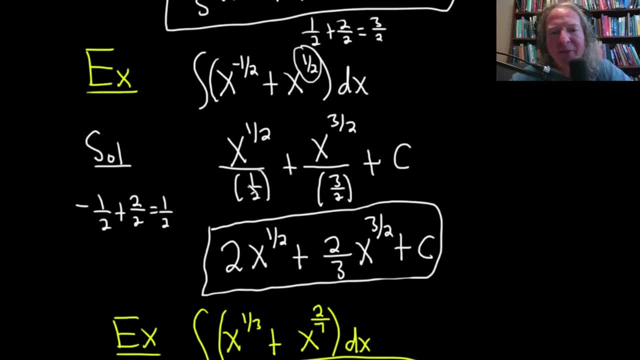 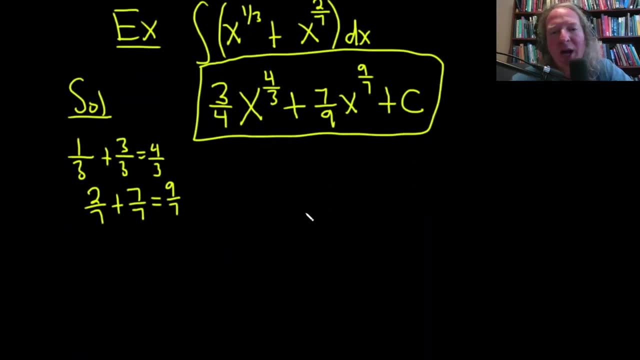 did that up here. right, We divided by one half, Here we divided by three halves, And then we flipped it when we multiplied by the reciprocal. So it's up to you whether you show those steps or not. Let's do another one. 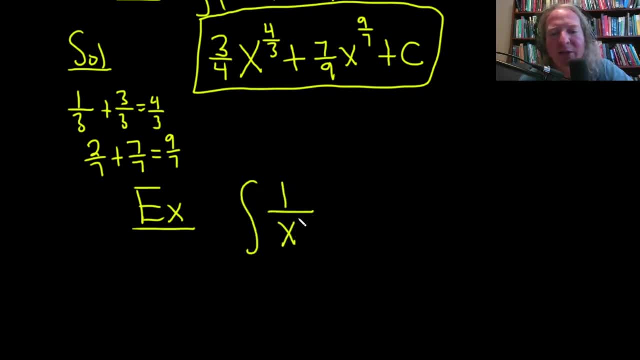 Let's do something like this a little bit simpler: One over x, cubed. So this is one where you can't just use the power rule right away. right, Remember, the power rule works on x to a power. Here we have one over x to a power, So what you have to do here is you have to rewrite. 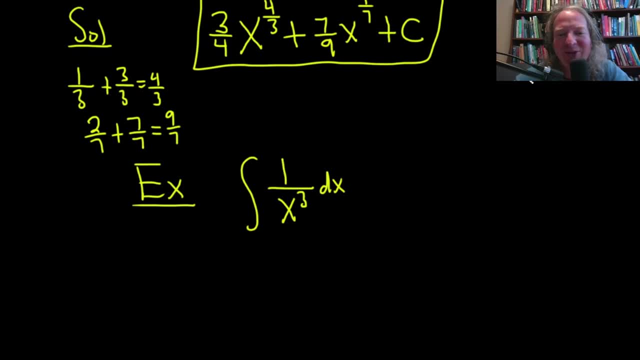 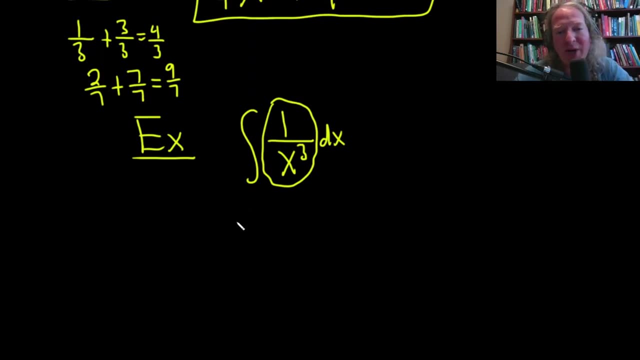 your integrand. See how good it is to have a name for that. So the integrand is this: here It's called the integrand, So we have to rewrite it. So because we're not integrating yet, we have to write the integral symbol. So, solution: So what we can do is we can bring this: 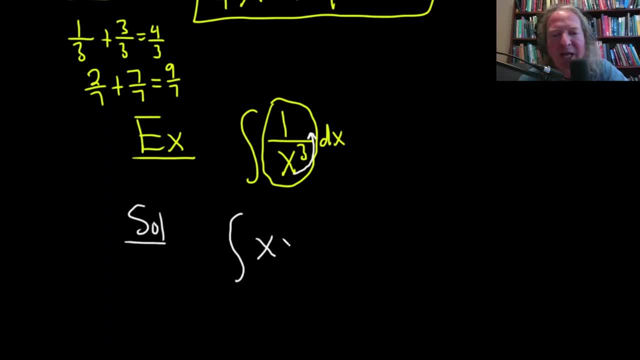 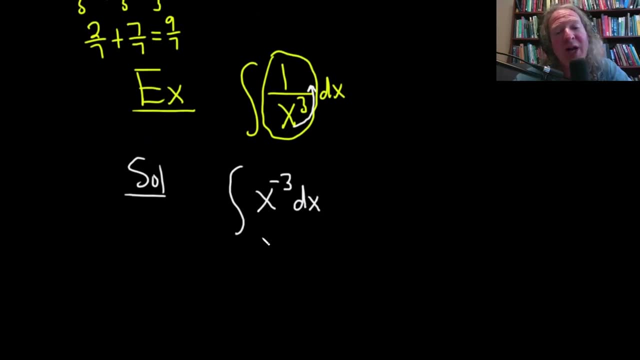 upstairs, And when we do that the exponent will become negative, So this will become a negative three. And then here we have a dx, And so now we can apply the power rule. So when we apply the power rule, we drop the integral sign, We take one and we add it to the exponent, So it'll be x. 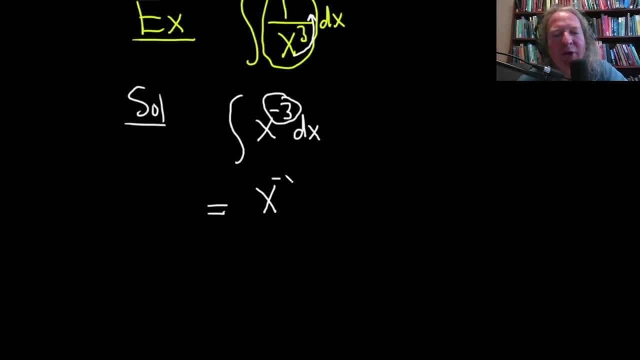 So let's see: Negative three plus two is negative three. One is negative two. Negative three plus one is negative two. Misspoke, We're adding one Negative three plus one is negative two And then you divide by negative two. 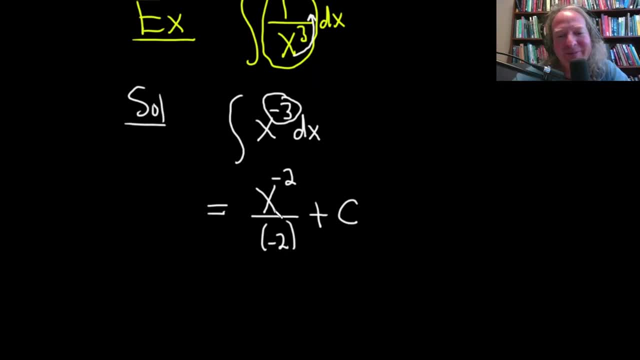 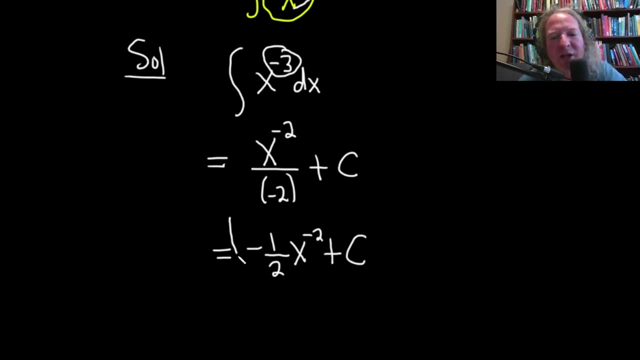 And then plus our constant of integration. Okay, This is equal to. So now what you can do here is you can write this as negative one half x to the negative two plus our constant of integration, b, And that would be a perfectly acceptable way to write the answer Some people would prefer to do. 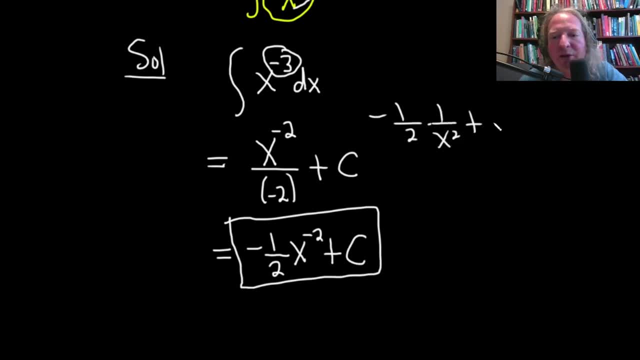 this. You could certainly do that, And you could certainly do something like this. I probably wouldn't do this. I'm not a fan. I prefer to do it this way, The easiest way, At least in my opinion. Okay, Let's integrate this. We have the integral of x cubed minus two, x plus four, all divided by x. 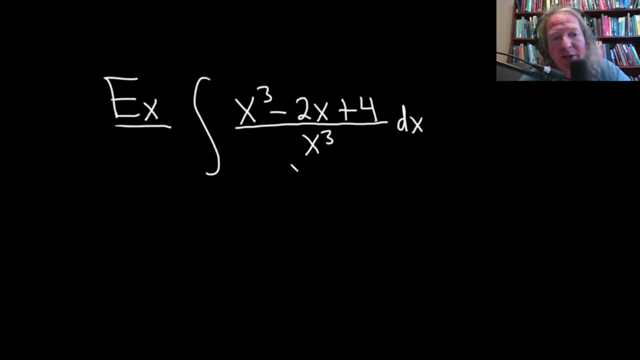 cubed, So we have a fraction, So let's go ahead and try to work through its solution. So, because we have a single term on the bottom, This is called a monomial. A good idea is to try to break this up into lots of little. 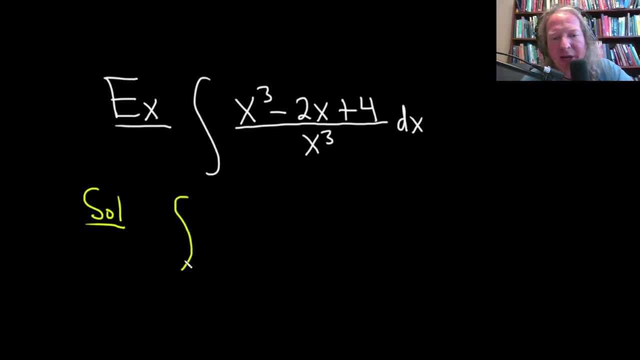 pieces. So we still have the integral sign, because we're not integrating yet, And so it'll be x cubed over x cubed, So x cubed over x cubed, And then minus, And then 2x over x cubed, So 2x over x cubed, So it's this over this minus, this over this, And 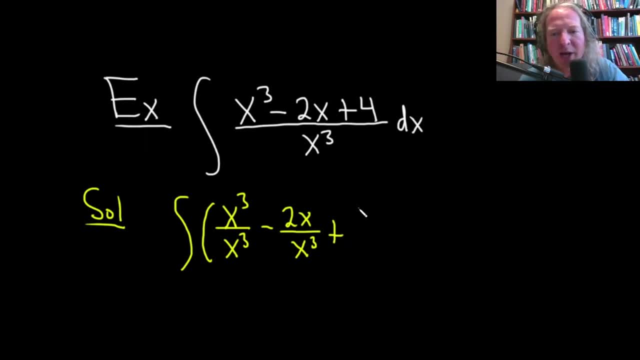 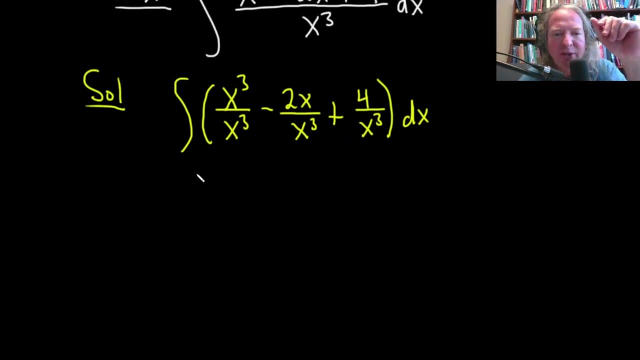 then plus And then four over x, cubed like that Boom. Beautiful, Really nice Parentheses. And then don't forget the dx. right, We still have to write the integral symbol and the dx until we actually apply some of our integration rules. So this is still the integral of: 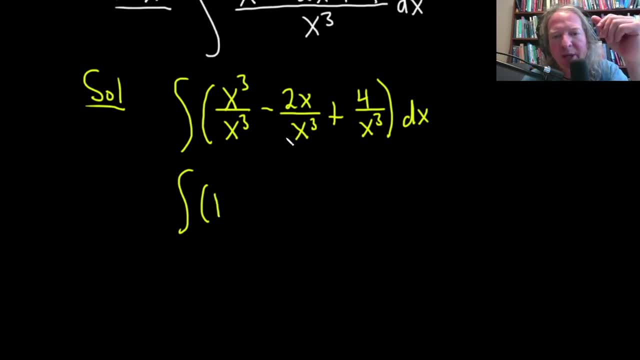 x cubed over x cubed is one Minus Here. we're going to cancel this x with one of these. That's going to give us 2 over x squared Plus, And then we have four over x cubed, And then we still have. 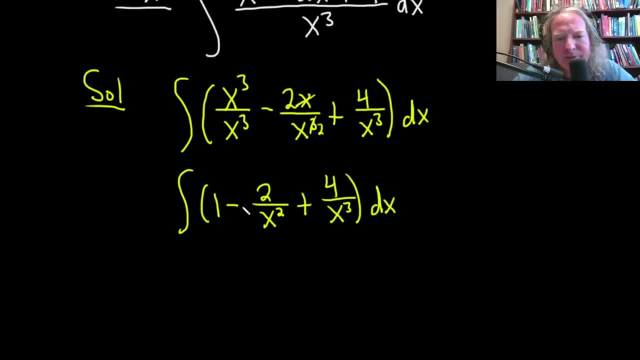 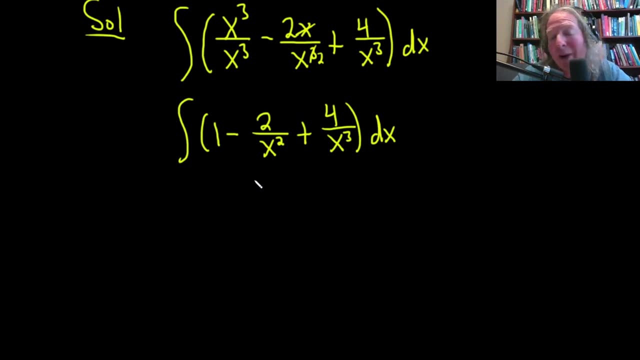 our dx. So in order to do this, we have to write it in a way that is doable. We have to write a power so we can apply the power rule. So what we can do is the one's. okay, We can take this and 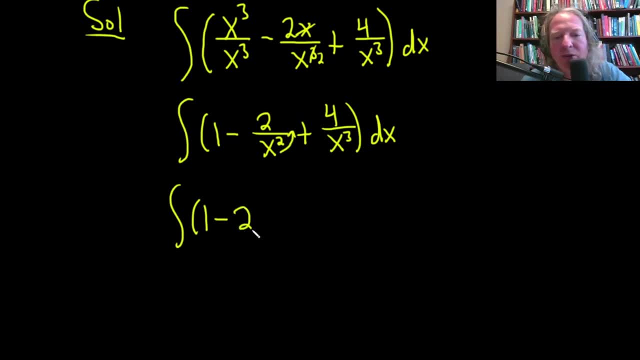 we can bring it upstairs. So this will be minus 2x to the negative 2, right, Because it becomes negative when you bring it up- And then plus 4x to the negative 3, like that, And then dx. Okay So. 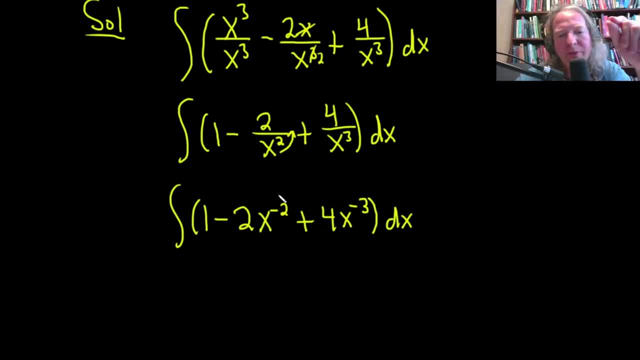 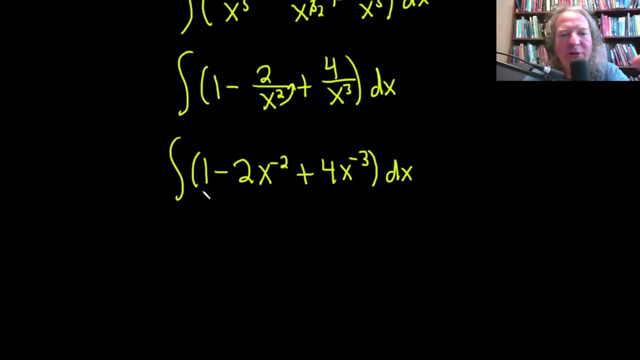 we have that in place where we can apply our rules. So now we're going to drop the integral sign, We'll drop the dx, So we're integrating 1.. Remember, if it's a number by itself, you just tack on the. 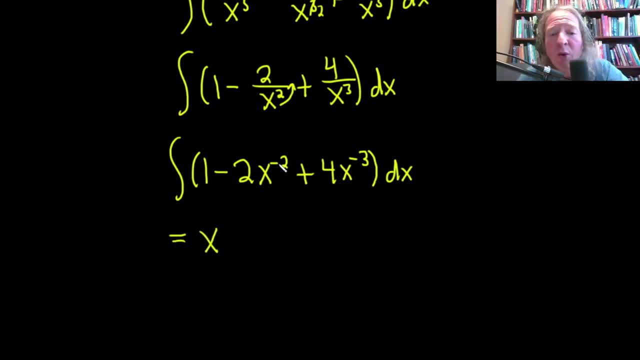 x. This will be x. Here we're using the power rule, So we're going to add 1 to the exponent here. So it'll be negative 2x to the negative. 2 plus 1 is negative 1.. And then we're dividing by negative 1.. 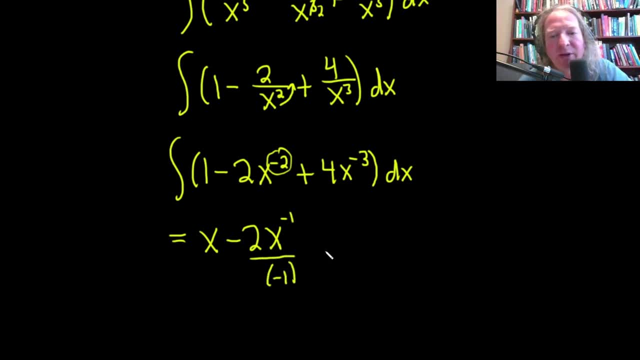 But you add 1 to the exponent and you divide by the result plus 4x to the negative. 3 is the exponent. We add 1 to the exponent, so it's going to be negative 2, right, Because 1 plus negative 3 is negative 2.. 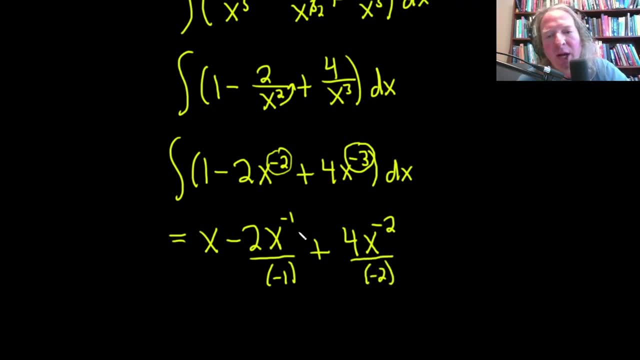 And then you divide by the negative 2. Got to be extra careful when there's negative numbers involved. It's very easy to get confused. We add 1, divide. add 1, divide plus C. It's really important to write the C, Even though. 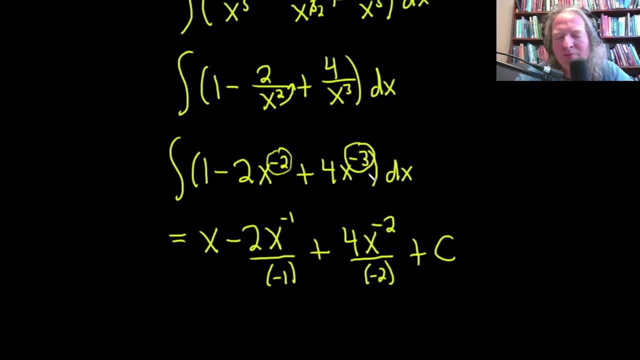 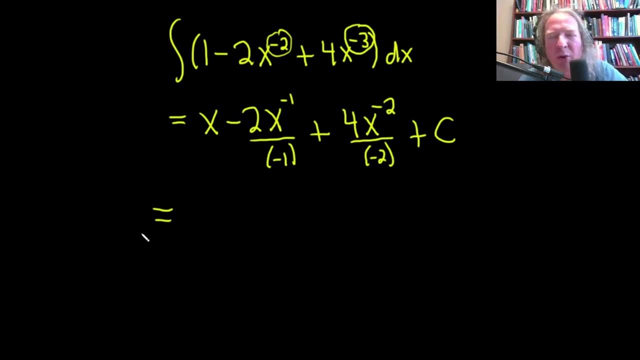 we're not done. once you integrate, you should most of the time- like 90% of the time- write it. I can think of like one example of an integration by parts problem where you don't really want to write it and it's kind of understood that you don't have to for various reasons. 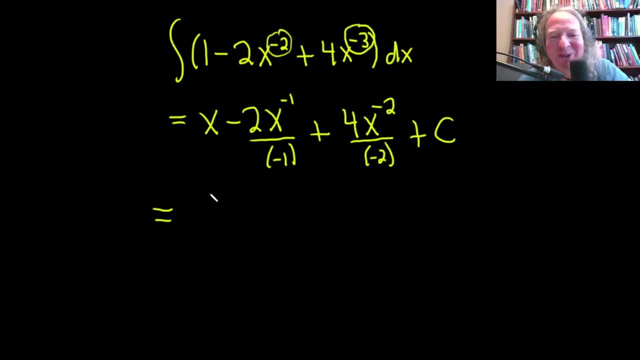 But for the most part you have to write the plus C. when you integrate These will become positives. This is x plus 2x to the negative, 1 minus. it's going to become a 2 here, minus 2x to the negative. 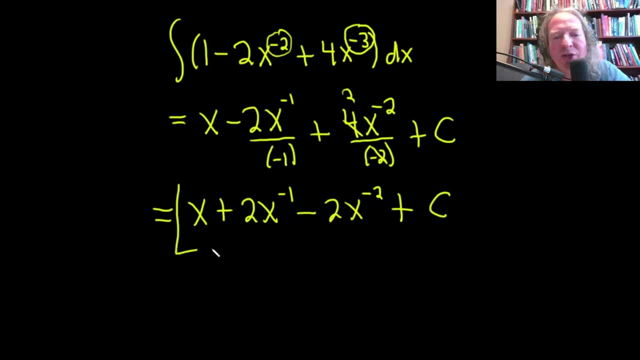 2. And then plus our constant of integration, capital, C, And you could leave it like this, or you could bring the numbers, the x's down, if you want. You could write it like this: x plus 2 over x minus 2 over x squared plus C. So if you, 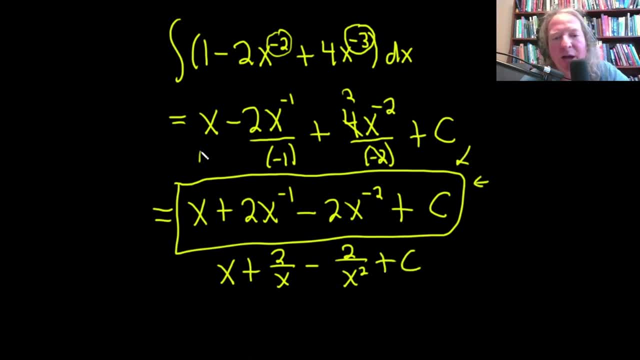 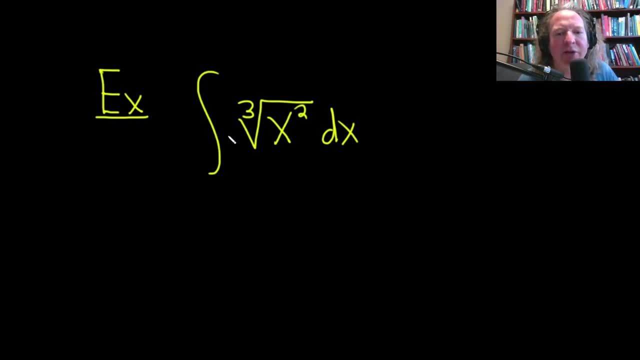 wanted to write it like this. you could. Personally, I prefer this. I think it's a much simpler answer. Okay, let's do this example: We have the integral of the cube root of x squared and we're integrating with respect. 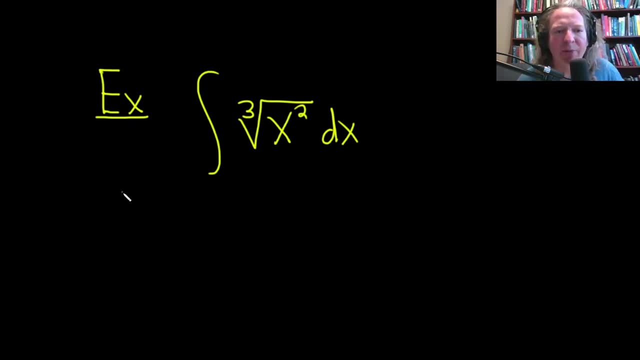 to x. So the trick for this problem is to rewrite it first. So because we're rewriting and we're not integrating yet, we still have to write the integral sign And basically this can be written as x to the minus 2.. 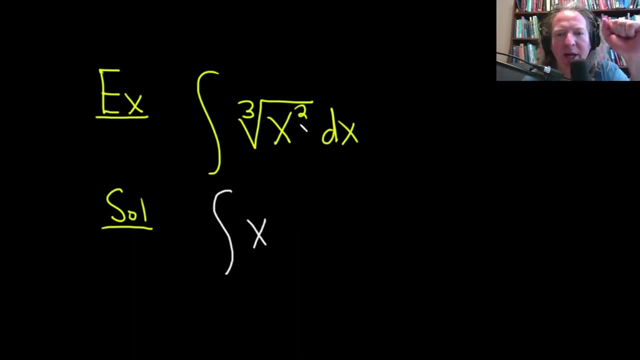 written as x to a power as follows: So it's x and it's gonna be this number here over this number. here, It's always this number over this number, So it'll be 2, 3rds, and then we have the dx. 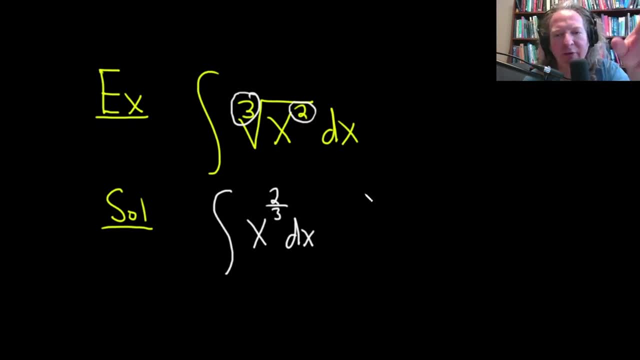 So again, it's always this number over this number. If you ever forget, just go back to the simple example of the square root of x. You might have this memorized as x to the 1 1⁄2.. And there's a 1 here and there's an implied 2 here. 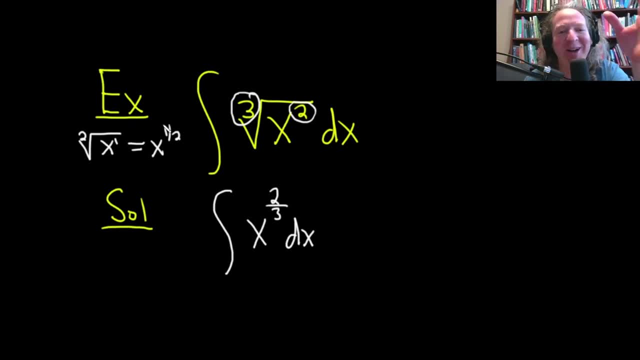 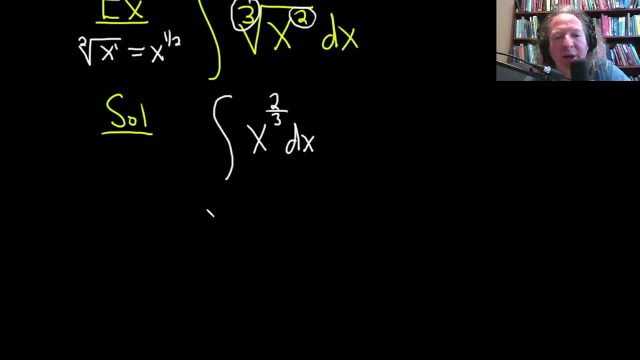 we can integrate using the power rule, But at this point we'll drop the integral sign, We'll drop the dx, and then it's x. And then, to figure out what goes here, you basically take this number and you add 1.. 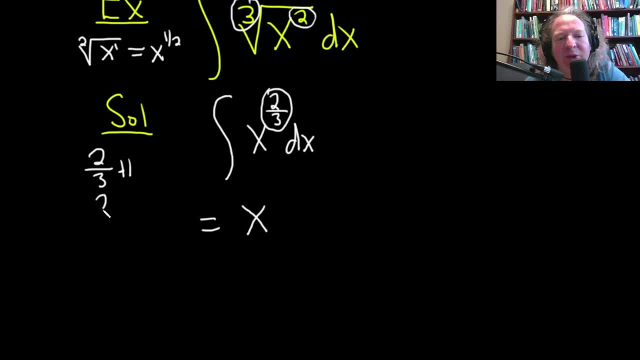 So it's 2 3rds plus 1.. That's really 2 3rds plus 3 3rds. That's gonna be equal to 5 3rds. So to the 5 3rds. 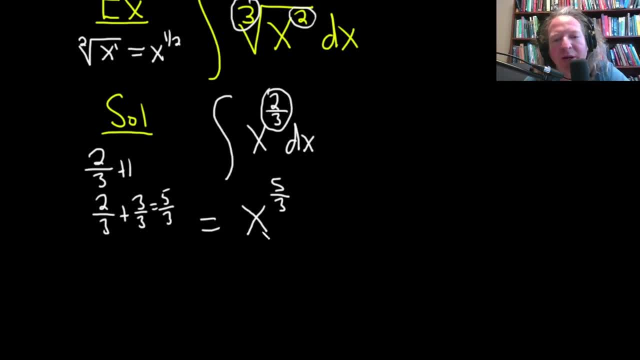 And then we divide by 5 3rds. right, The rule says you add 1 and then divide by 5 3rds, And then you add your constant of integration capital C. So you add 1 to this, write the result and divide. 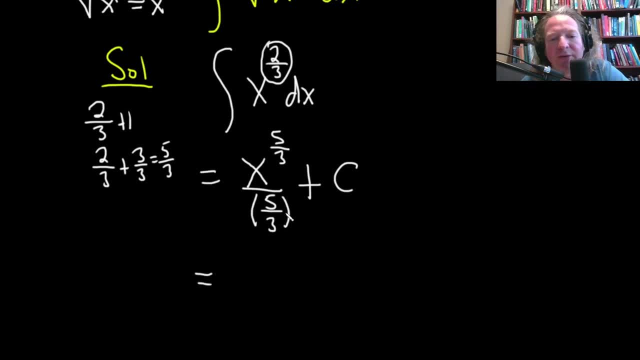 And I could have skipped this step. Remember, when you divide by a fraction, you're really multiplying by the reciprocal. So it's really 3 5ths, x to the 5 3rds, and then plus our constant of integration capital C. 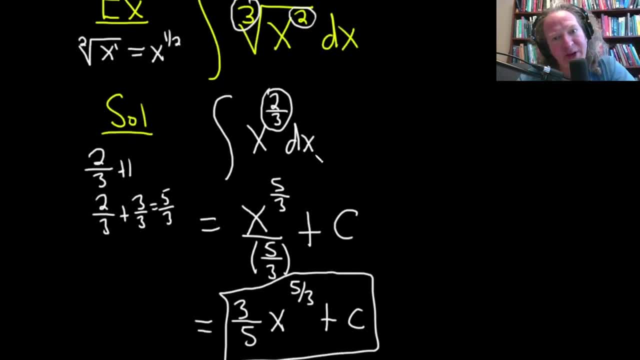 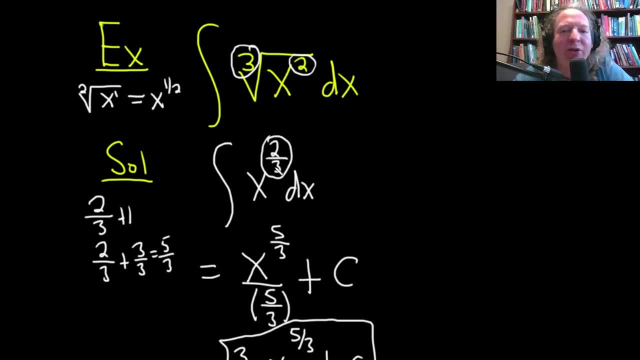 So pretty simple. Again, the key step, I think, is start off by rewriting it So it's this number over this number, And then just apply the power rule when you get here. So you take the 2 3rds and you add 1 to it. 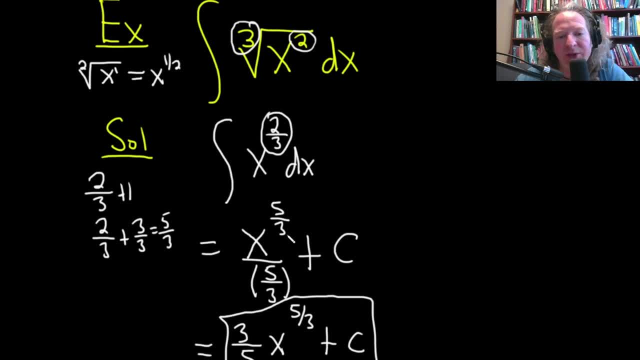 So 2 3rds plus 1 is really 2 3rds plus 3 3rds, which is 5 3rds, And then you divide by 5 3rds, but that's the same thing as multiplying. 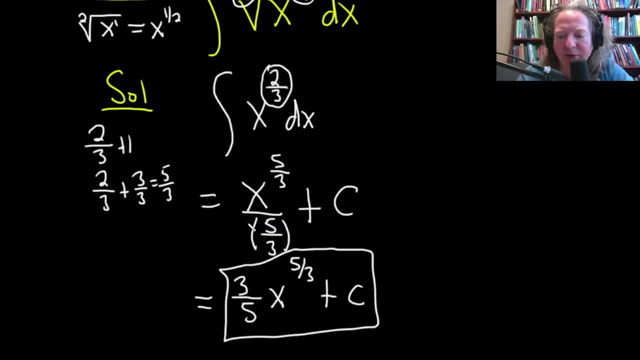 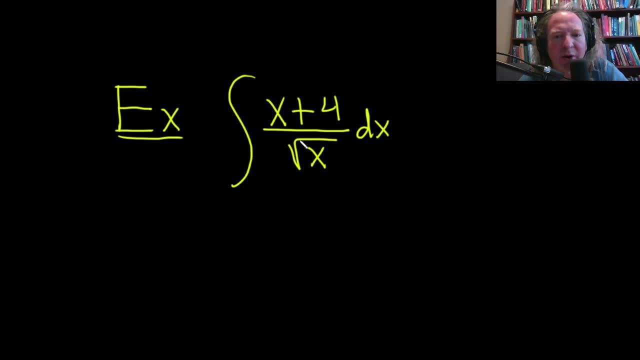 by the reciprocal of 5 3rds, which is 3 halves. Okay, in this example we're going to integrate x plus 4 divided by the square root of x. So let's go ahead and try to work through this one solution. 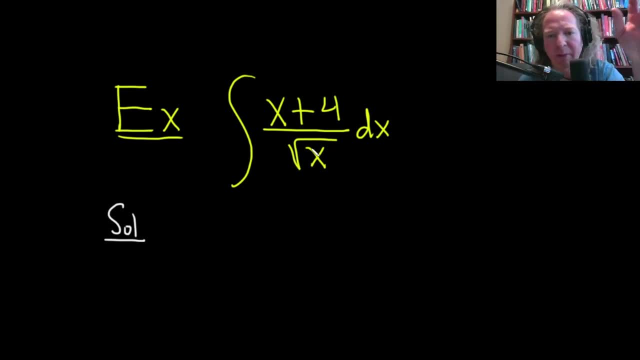 So because we have a single term on the bottom, it's called a monomial. what we're going to do is we're going to break this up into two pieces. Also, I want to emphasize that- the square root of x- we can think of this as x to the 1 half- 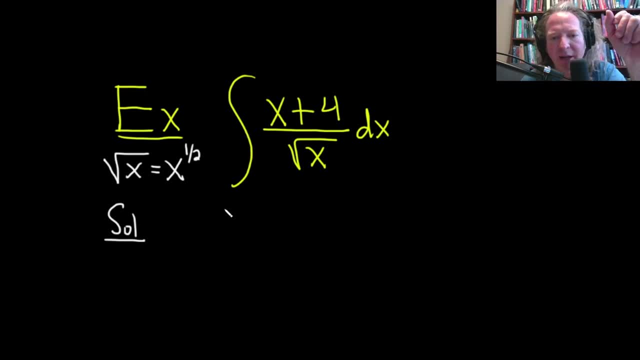 super useful to know. So let's go ahead and break it up And at the same time we're going to think of the square root of x as x to the 1 half. So it's going to be this over this, It'll be x over, and then x to the 1 half. 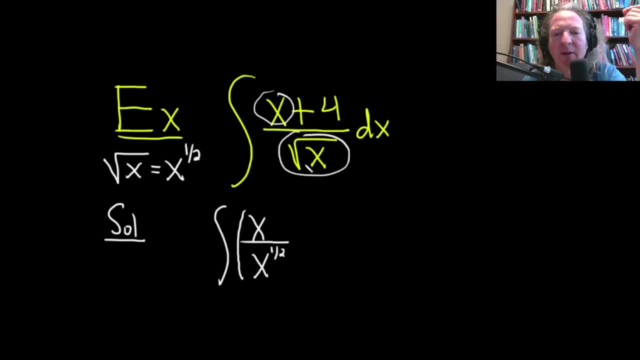 And then parentheses plus, and then 4 over, and again x to the 1 half, just like that, And then dx. Okay, so, just breaking it up, it's x over the square root of x, but that's really x to the 1 half. 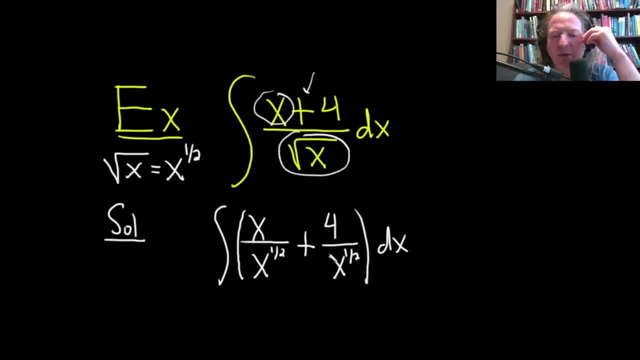 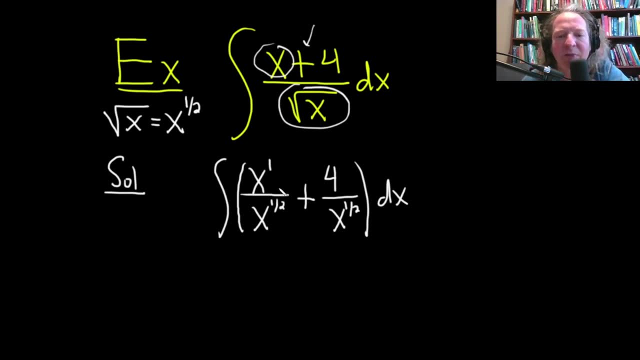 Plus 4 over the square root of x, but that's really x to the 1 half. All right, there's really a 1 here. So whenever you have something like this, you basically subtract the exponents, Recall if you have, say, x to the m over x to the n. 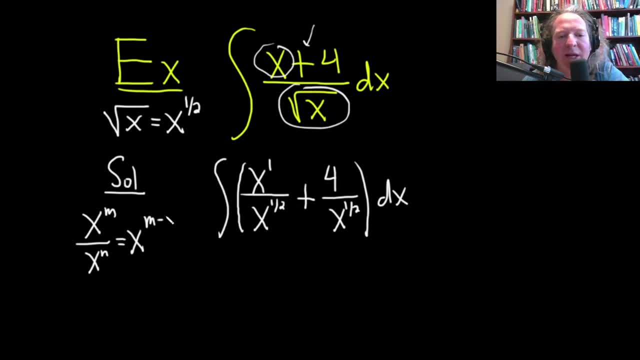 that's equal to x to the m minus n. So you basically just subtract here. so it's the integral sign And we haven't integrated yet, right? So we still have to write this. We don't have to write the integral sign. 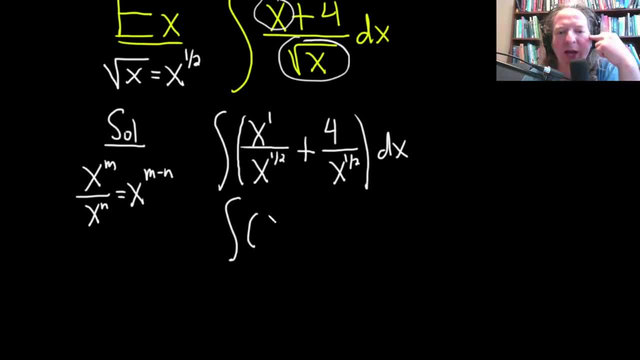 We still have to write the dx. So 1 minus 1 half is 1 half. And then here what we'll do is we'll bring this upstairs, And when we do that, we get 4x, So the exponent will become negative. 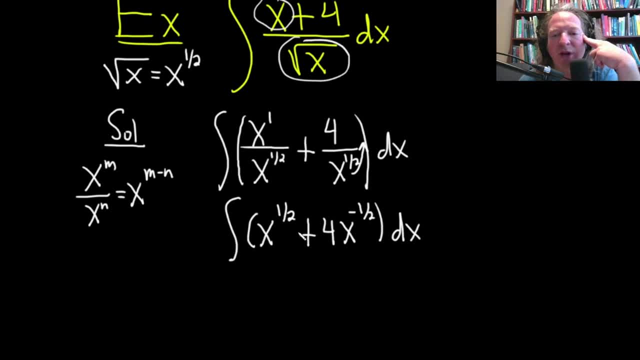 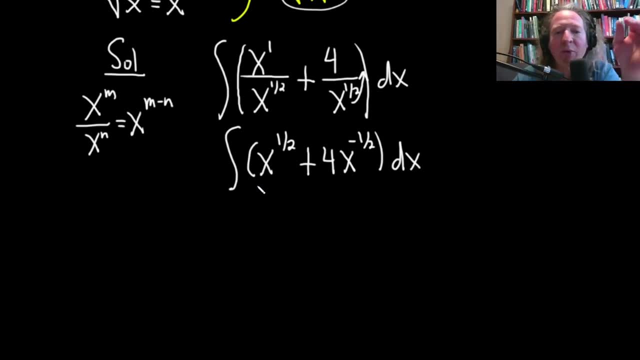 So it'll be negative 1 half. And we've done these things because we want everything to be x to a power, so we can use the power rule. So now we're going to go ahead and integrate. This is equal to, And when we integrate, we drop the integral sign. 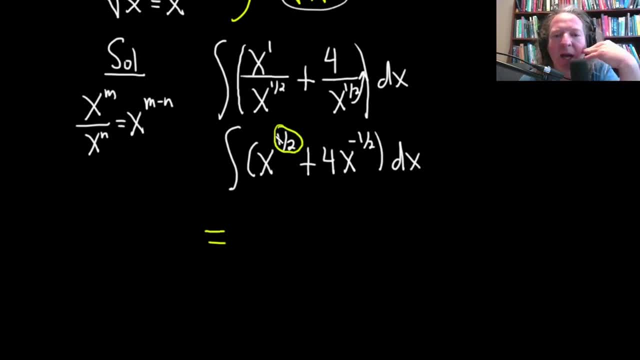 We drop the dx, So we take this exponent here and we add 1 to it. So 1 half plus 1 is going to be 1 half plus 2 halves, so 3 halves. So this is x to the 3 halves. 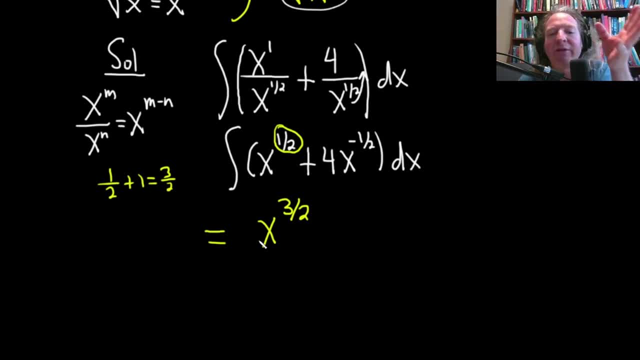 And then we're supposed to divide by 3 halves. But instead of dividing by 3 halves we can always multiply by the reciprocal, So 2 thirds plus 4.. I'm going to leave some room here, And this is x. 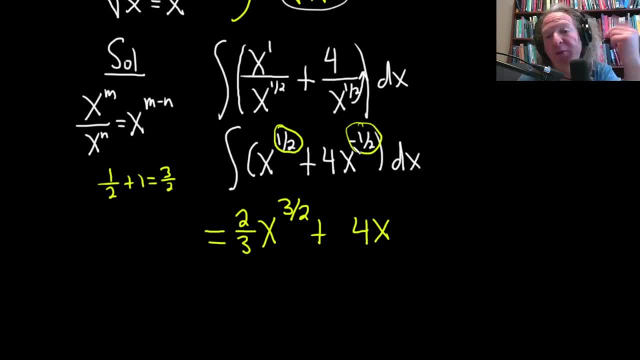 We add 1 to the negative 1 half, So that's 2 halves plus negative 1 half, So that's 1 half. And then dividing by 1 half is the same thing as multiplying by 2 over 1.. And then plus our constant of integration capital C. 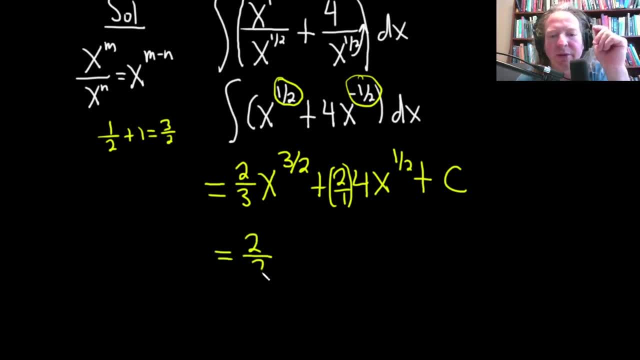 So this is equal to: let's see: 2 thirds, x to the 3 halves, And then 2 times 4 is 8.. So this is going to be 8x to the 1 half, plus our constant of integration capital C. 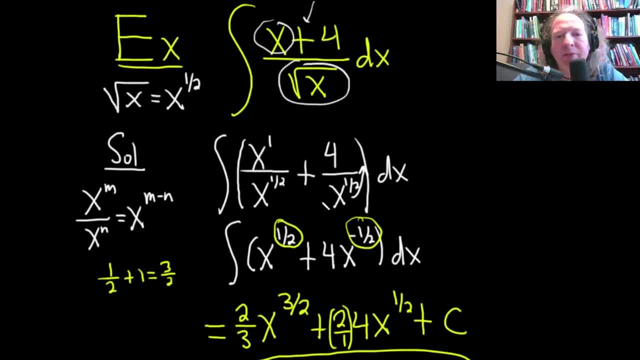 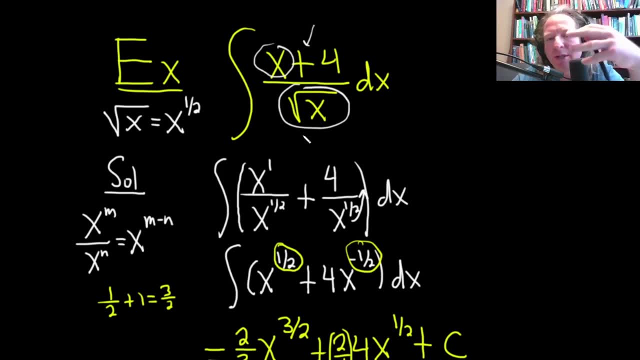 So just a quick recap: When we first saw the problem, when you see something like this, when you see a single term on the bottom like this, you should be thinking, hey, can I break this up? Is it a possibility? Can I do that? 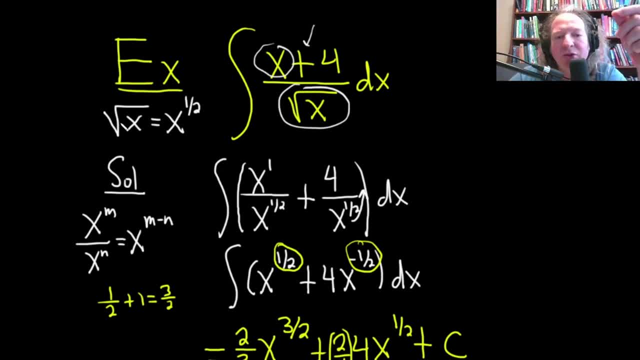 Yes, Yes, you can, Let's do this. Let's do this over this: Square root of x is really x to the 1 half. So we did that Here. we just did some algebra: 1 minus 1 half is 1 half. 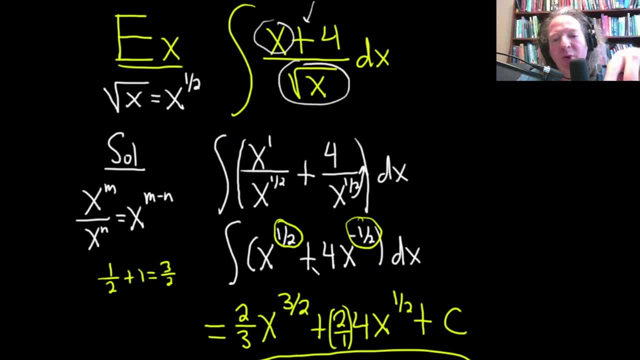 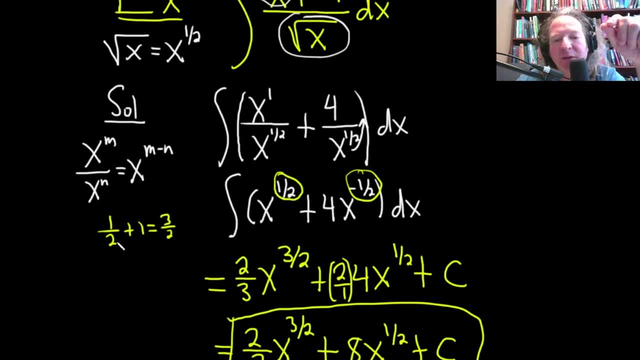 We brought this one upstairs, It became negative. At this point everything is x to a power, And so we can actually apply the power rule. So we just basically add 1 to each of the exponents. 1 half plus 1 is really 1 half plus 2 halves. 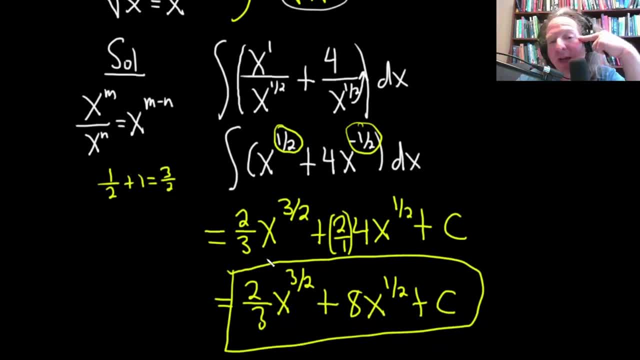 which is 3 halves, And you're supposed to divide by 3 halves. But instead of dividing by 3 halves, we chose to multiply by the reciprocal, which is 2 thirds. Same thing here: We're supposed to divide by 1 half. 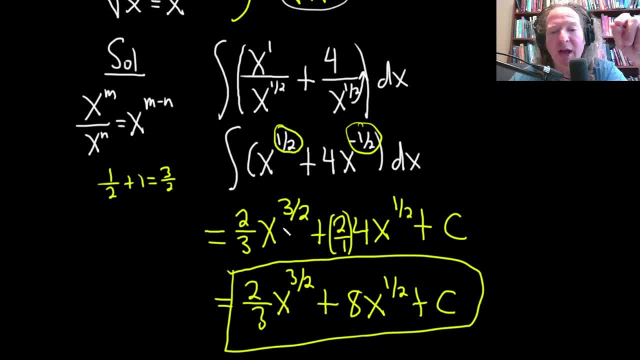 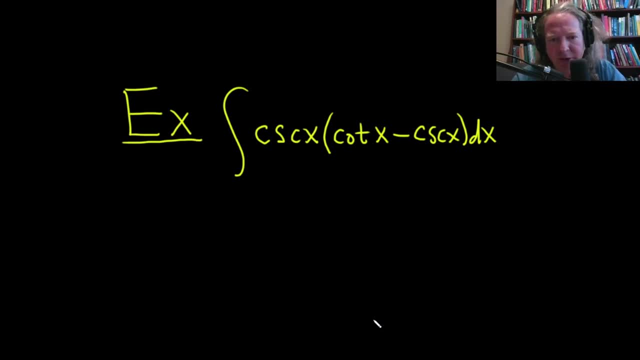 Instead, we multiplied by the reciprocal, which is 2 over 1. And then just cleaned it up: 2 times 4 is 8. And all is good. OK, let's work out this indefinite integral. We have the integral of the cosecant of x. times cotangent of x minus cosecant x. We have a product here, So we need to figure out how to do this. So one idea is to make sure that we maybe just distribute the cosecant and see what happens. So we still have the integral sign. 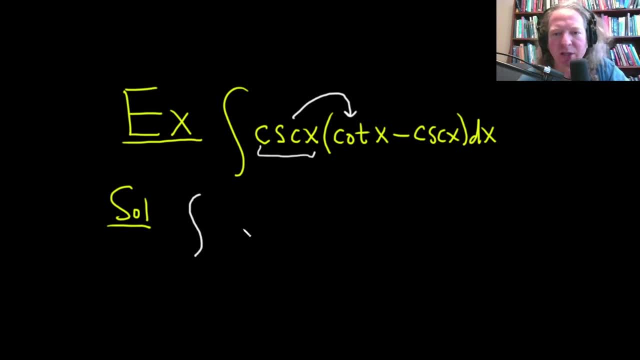 And so now we're going to multiply cosecant times cotangent. It's going to give us cosecant x, cotangent x. And then cosecant times: negative cosecant is negative, cosecant squared x. Really nice, Really really nice. 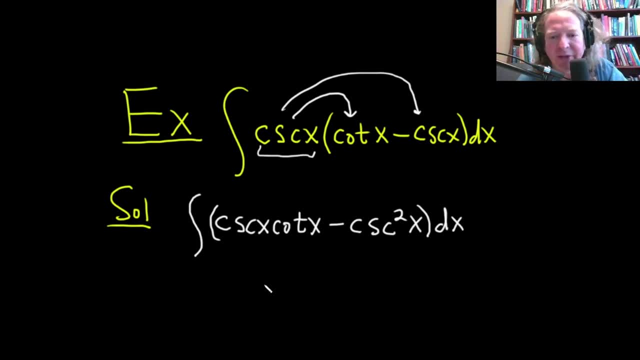 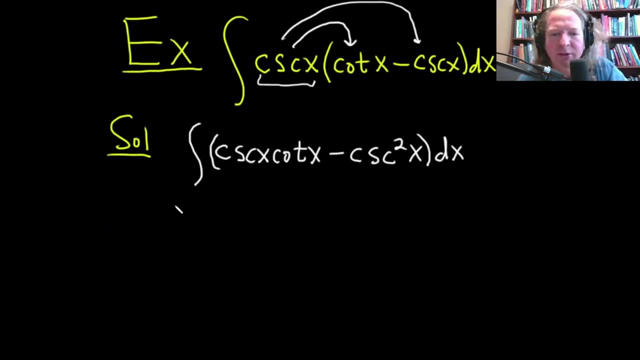 And this is dx. We have our little dx there, And so now we should be able to integrate this using some formulas. So this is equal to, So let's integrate cosecant cotangent. So when you're trying to do that, 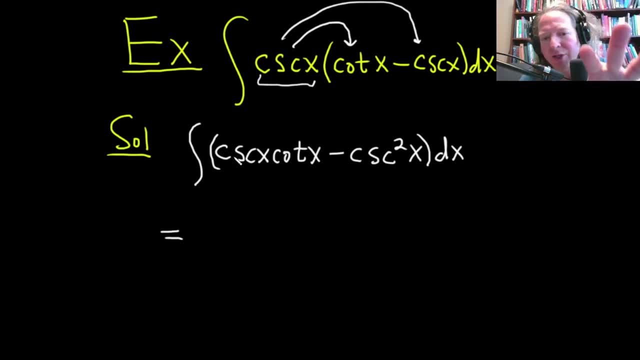 the question you want to ask yourself is: what is a function whose derivative is cosecant cotangent? Well, the derivative of cosecant is negative cosecant cotangent. So here, if you put a negative cosecant of x, 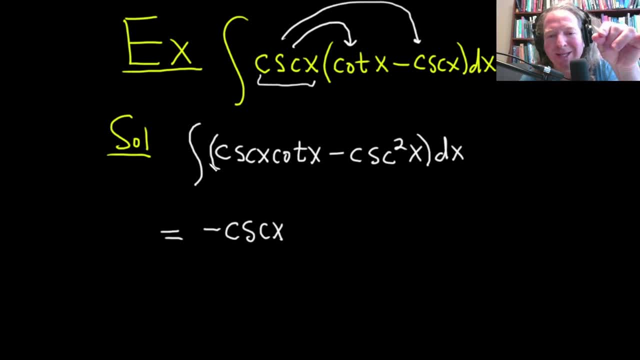 all is good, Because the derivative of cosecant is negative: cosecant cotangent. We already have a negative here. The two negatives are going to make this a positive. And then here, what's a function whose derivative is cosecant squared? 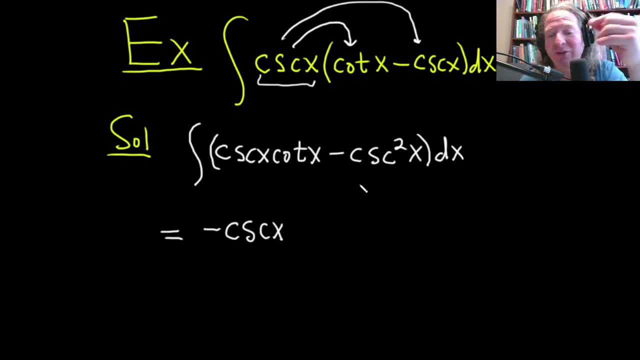 Well, the derivative of cotangent is negative cosecant squared. So this is going to be a plus cotangent of x, And then we still have our plus c, which is our constant of integration. So that worked out really nice. Let's just double check it. 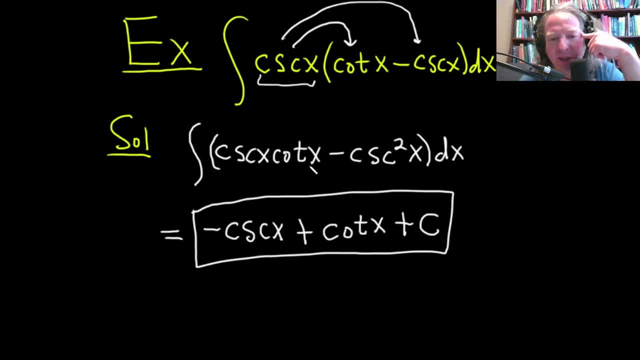 The derivative of cosecant is negative- cosecant cotangent. But we've already got a negative here, so that's going to make this positive. And then the derivative of cotangent is negative- cosecant squared. So that works out, you know. 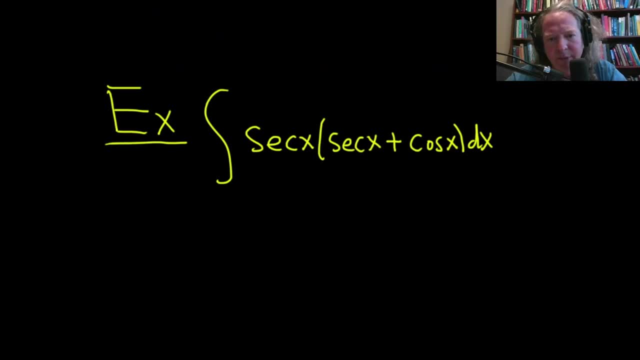 super perfect in this example. Okay, let's go ahead and try to integrate this. We have the integral of secant times, secant of x plus cosine of x. So to do this, a good first step might be to just distribute the secant. 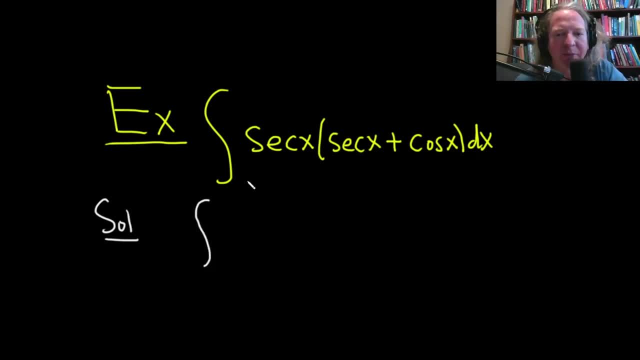 and see what happens. So we have our integral sign here, And then secant times secant, that's going to be secant squared of x, And then plus secant times cosine is going to be secant times cosine, And then we have our dx here. 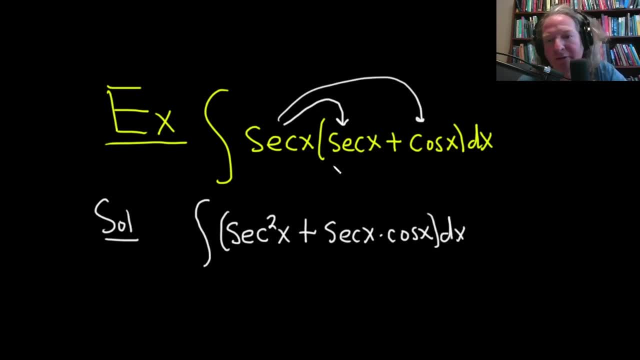 So just start off by distributing, because we don't really have, you know, an easy way to just immediately do this problem. So it's a good. first step is to just take this and multiply it by each of these, So we need to think about each piece here. 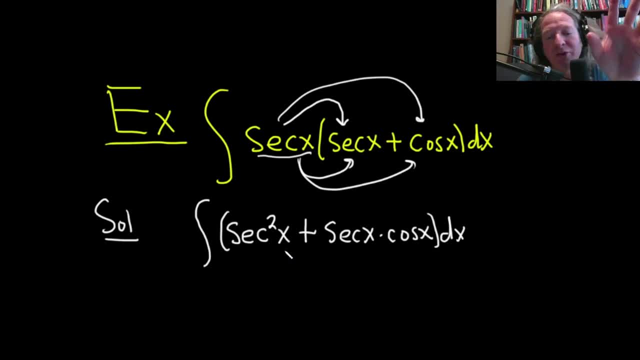 before we proceed. So the derivative of tangent is secant squared. So when we integrate secant squared we're going to get the tangent function. So that's pretty simple. But this secant cosine, there's not really a nice formula here. 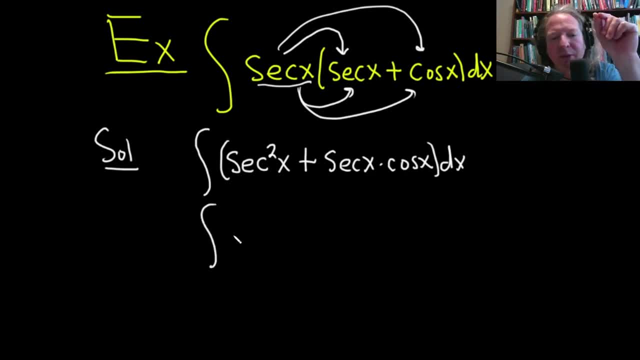 except- you might recall- this is the key here- this is secant squared x plus secant is really 1 over cosine. So this is 1 over cosine x times cosine x. So it works out really, really nice here, because they cancel right. 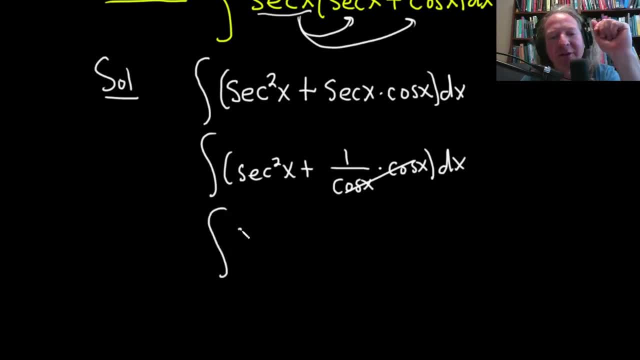 It's going to give you 1.. So this is going to be the integral of secant squared. Secant squared x plus 1.. Beautiful, right, dx? What a cool problem. Yeah, so just a little thing there. Just you know, keep in mind. 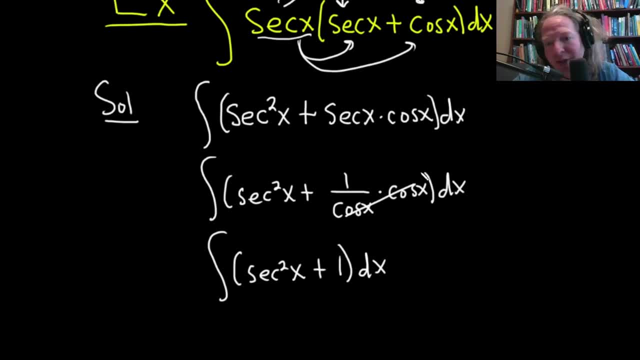 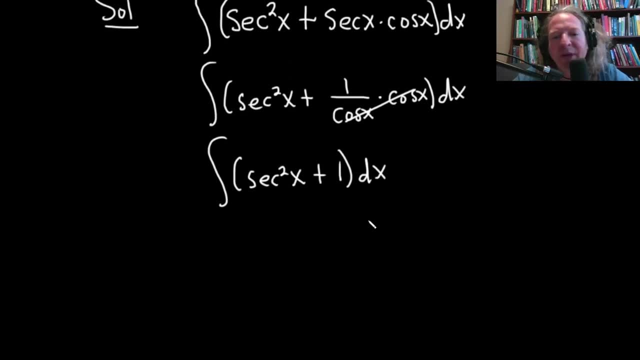 these are reciprocals of each other. Likewise, cosine is 1 over secant, So you could have done it that way too, And the secant would have canceled. That would have been a perfectly acceptable way to do it. So now we're integrating. 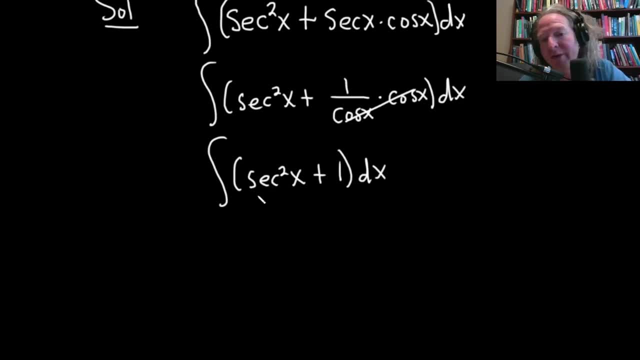 So let's think backwards again. What's a function whose derivative is secant squared? Well, tan x. Right, The derivative of tangent is secant squared, And to integrate 1, since it's a constant by itself, you just tack on an x. 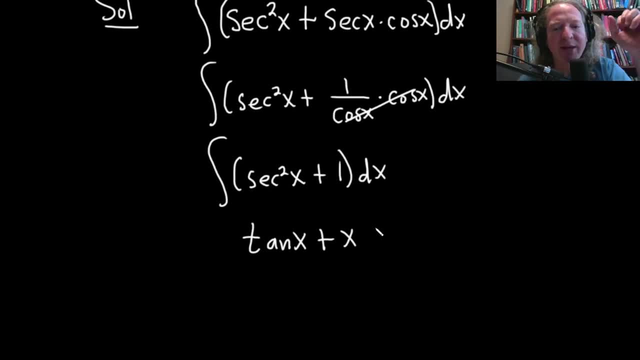 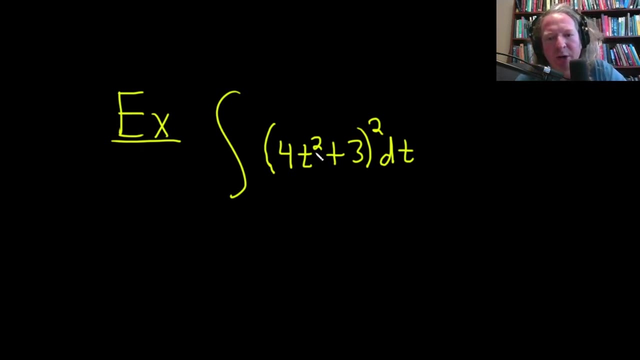 So it's just x And it's not quite right. yet We still need our constant of integration capital C. That would be a perfectly acceptable answer to this problem. Okay, in this example, we're going to integrate 4t squared plus 3.. 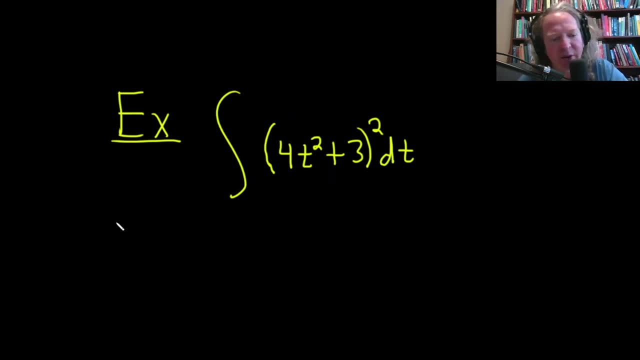 And then the whole thing here is being squared. Let's go ahead and try to work this out. So let's go ahead and write the solution. So to do this, I think one way to do it is to simply expand it out, And because there's a 2 here, 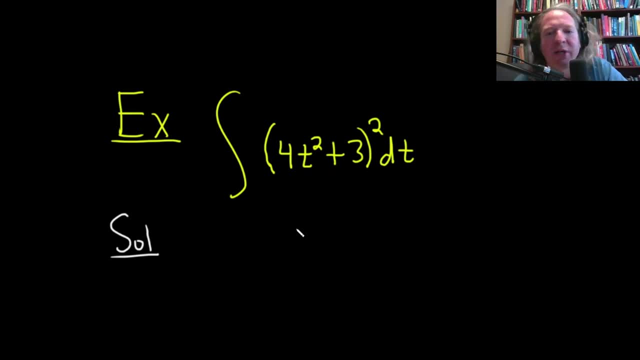 you can write it twice and just multiply it out. Or you can take a shortcut. Let's go ahead. and how should we do it? Oh, let's just write it twice. So this is going to be 4t squared plus 3. 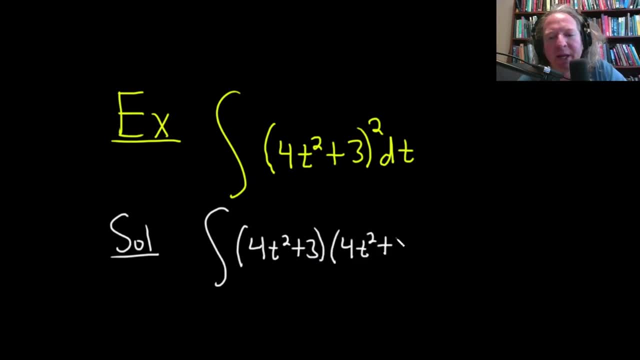 times 4t squared plus 3.. And then what we can do is basically distribute and then apply the power rule. If you're curious about the shortcut, I was going to apply the formula a plus b squared, That's equal to a squared. 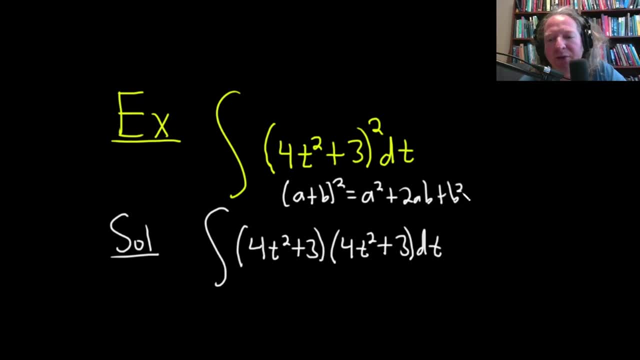 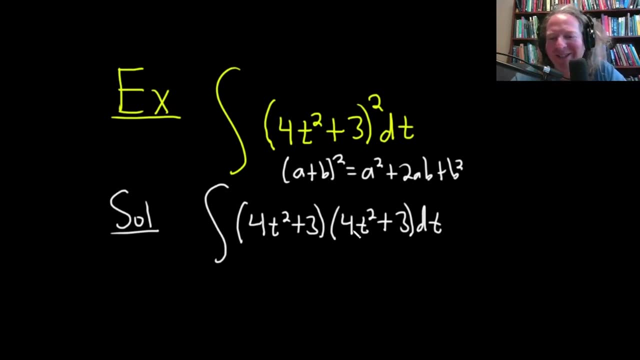 plus 2ab plus b squared, So you can apply this formula to this here, And it's a little bit faster to do it that way, But we've started doing it this way, So let's just continue. All right, good stuff. 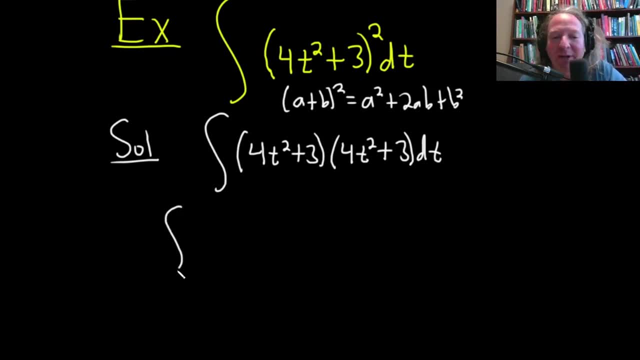 So we're not integrating yet, So we still have to write the integral sign. So we're going to do this times this. So that's going to give us: let's see: 4 times 4 is 16.. t squared times t squared. 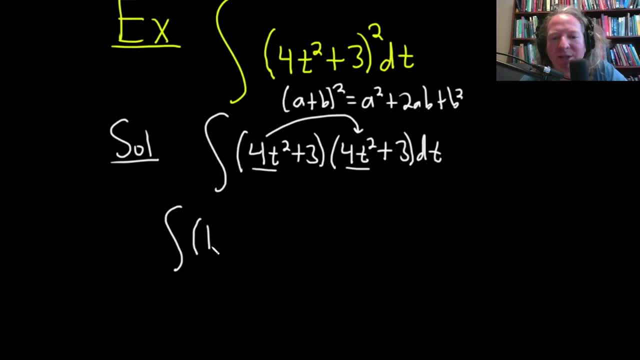 is t to the fourth, So that'll be parentheses 16t to the fourth Right. And then we'll do this times this: That's going to be 12t squared. Yeah, really nice. And then this times, this is also going to be 12t squared. 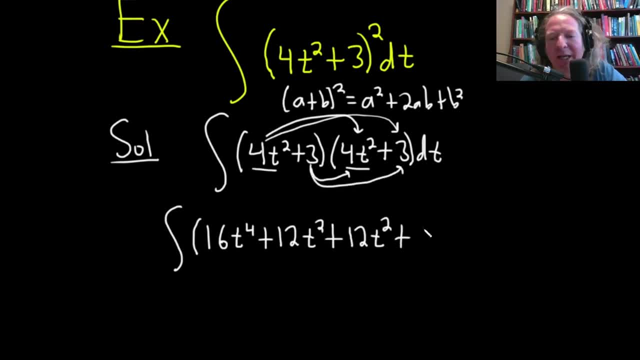 And then, this times this is going to be 9.. And then we have the dt. So basically, you take this number- here This is a different color, This expression, here 4t squared- And you multiply it by both of these. 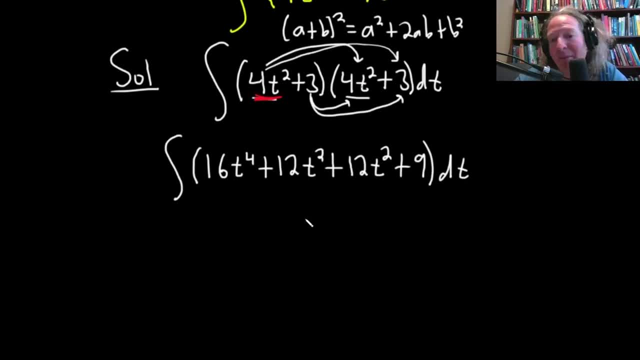 And take this term here and multiply it by both of these. All right, Looks like we can combine some like terms, So let's do that. So this is going to be the integral of 16t to the fourth, And then we have 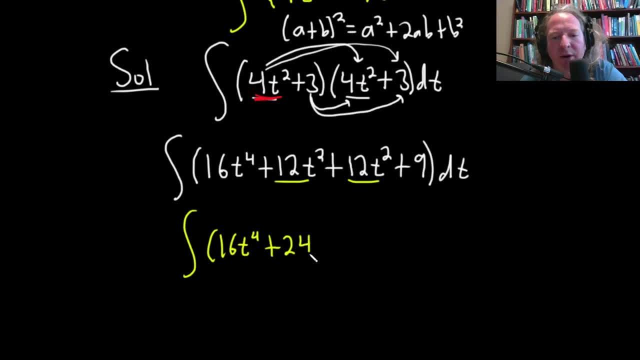 12t squared plus 12t squared, That's going to be 24t squared. Right, 12 is 24.. And then plus our 9 here dt- Really cool, All right. So now we can just apply the power rule. 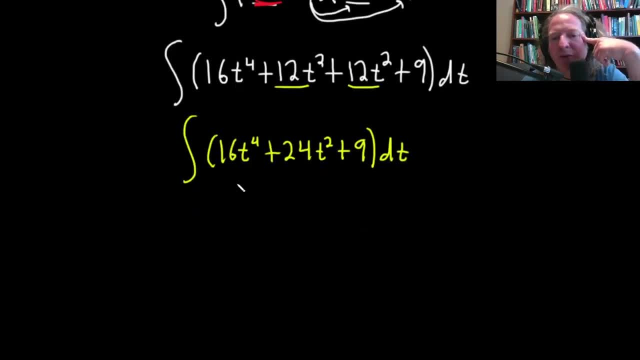 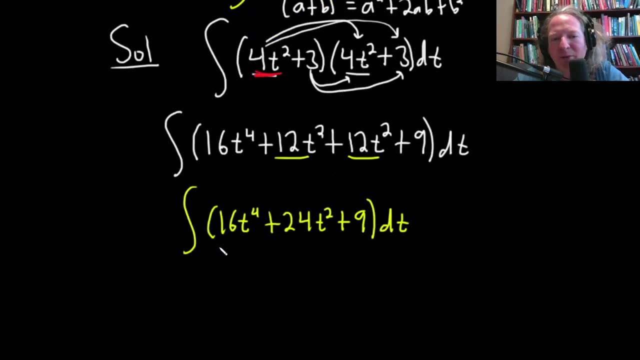 So let's do it. So when we integrate, that's when we drop the integral sign, Right? It's really important. So you notice it's written every single time, Right? At this point we stop writing it, Okay. 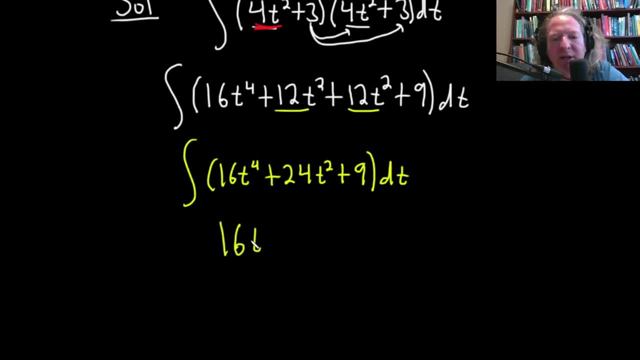 And so this is going to be 16t to the 5.. Okay, And then you just divide by the number Right. You just basically take this and add 1.. 4 plus 1 is 5.. Then you divide by the result. 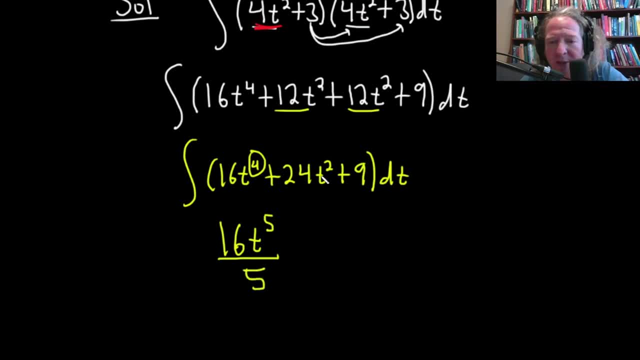 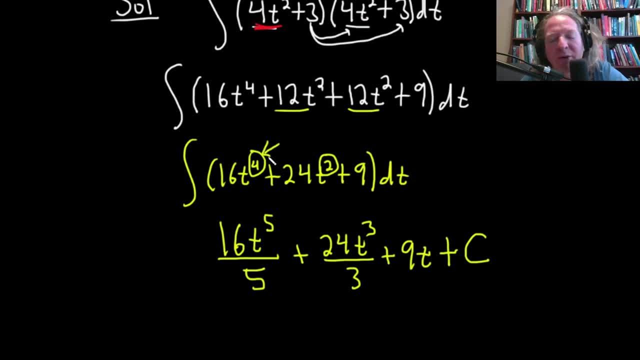 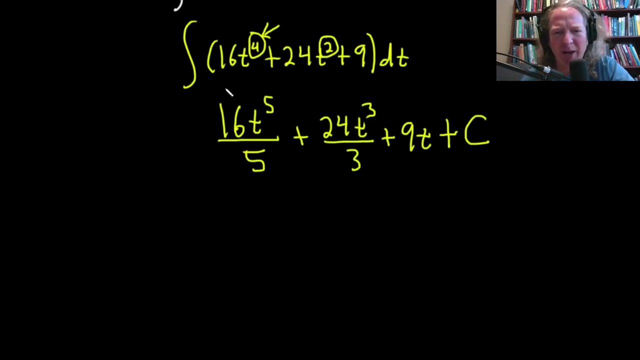 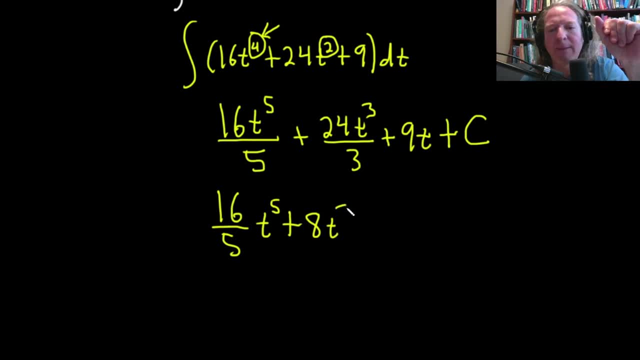 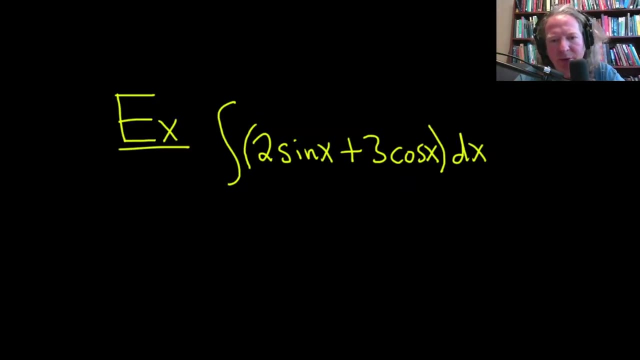 8 times. this is 8 t cubed and we have the 9 t. very nice. and then we still have our constant of integration, which is capital c, and that would be the answer to this integral. in this example, we're going to integrate two times the sine of x plus three times the cosine of x. let's go ahead. 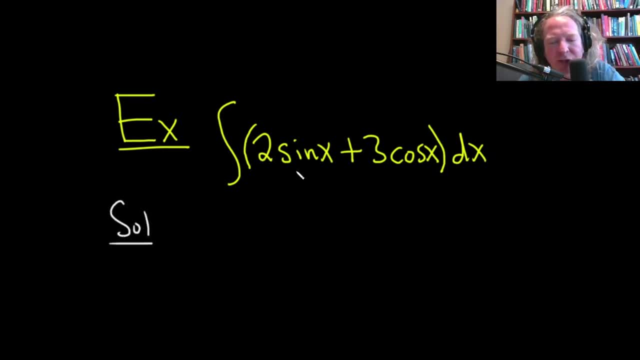 and work through its solution. so we should be able to just jump into it and work it out right away. so let's try to think backwards. first of all, note that the constants in front of the trig functions, they're just going to hang out. so this is two. 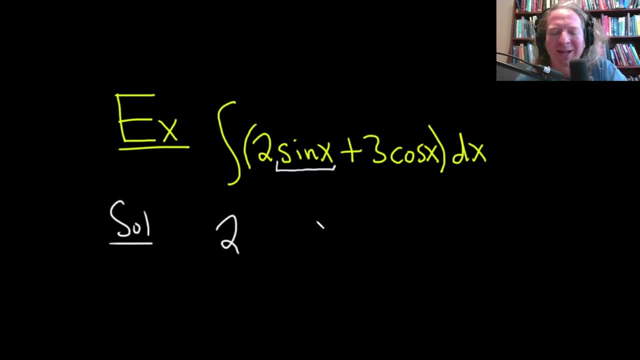 you and then we're integrating sines. so what's a function whose derivative is sine? well, the derivative of cosine is going to give you negative sine. so if you take the derivative of negative cosine, it'll be a negative, negative sine, which is a sine, so it's going to be negative cosine. i'm going to put the negative here out front. let's check that. 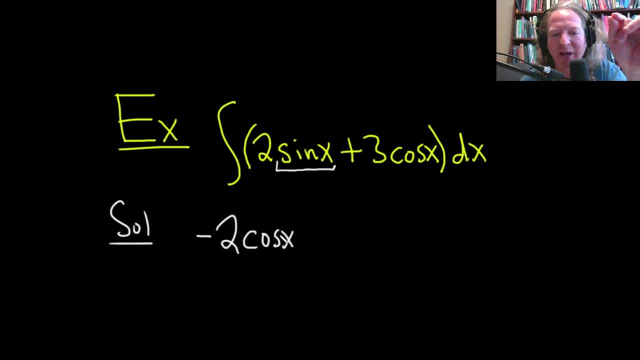 if we take the derivative of cosine, we get negative sine. there's a negative two here, so that's going to give us 2 sine x. And then here we're looking for a function whose derivative is cosine. Well, the derivative of sine is cosine, so this will be plus 3 sine x, plus our constant.